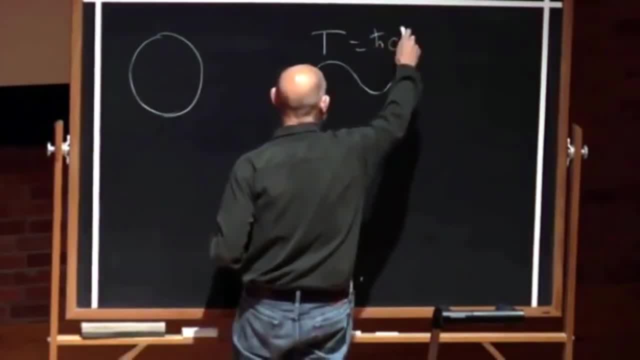 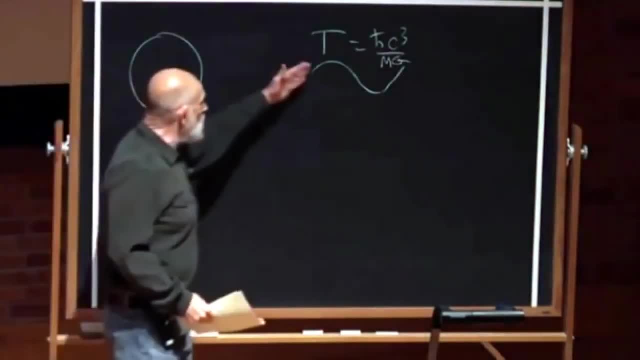 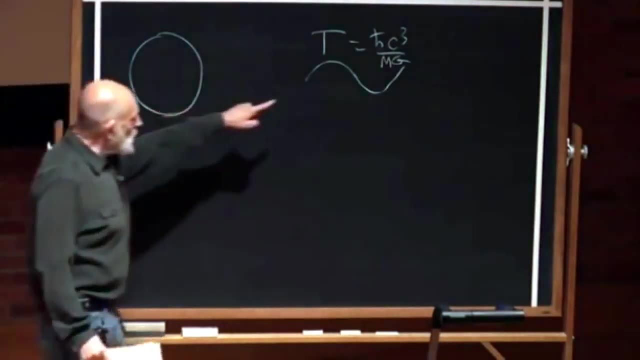 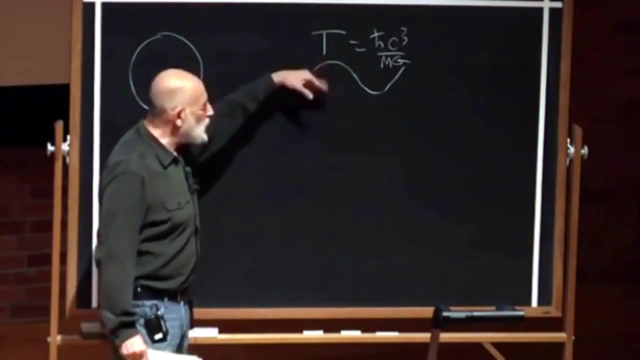 whatever it is- h bar c cubed over mg Associated with. that is an energy for each photon. The photons have about that wavelength and they just fly out, But a photon that appears over here with this temperature, it's also the energy of the photon, Temperature and energy. 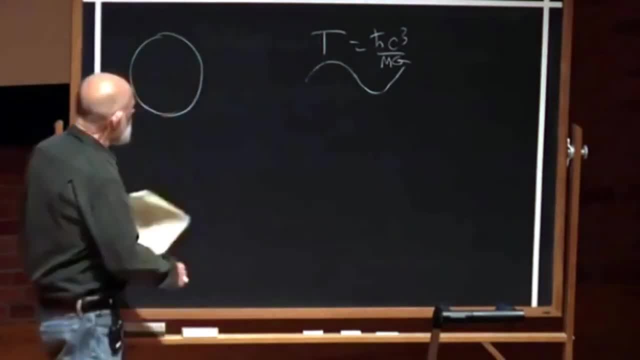 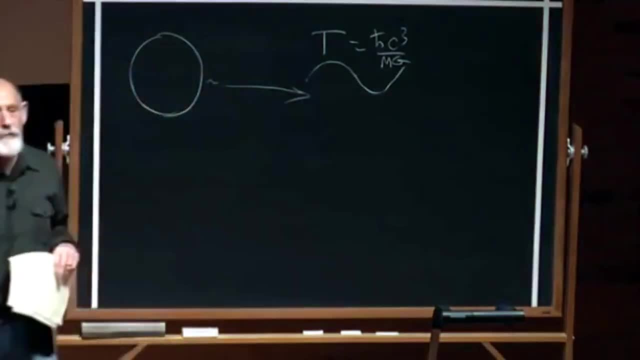 are roughly related. This is also the energy of the photon. When a photon materializes at the horizon and goes out, it loses energy. Why does it lose energy? For the same reason that if I threw this chalk up in the air as it rises. 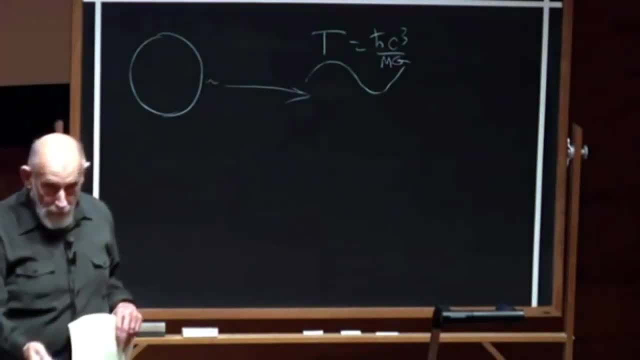 it loses kinetic energy. The gravitational field is pulling it back and the result is that it loses kinetic energy. The same thing happens to the photon: as it goes out, It loses kinetic energy, But by the time it gets out it has this much. 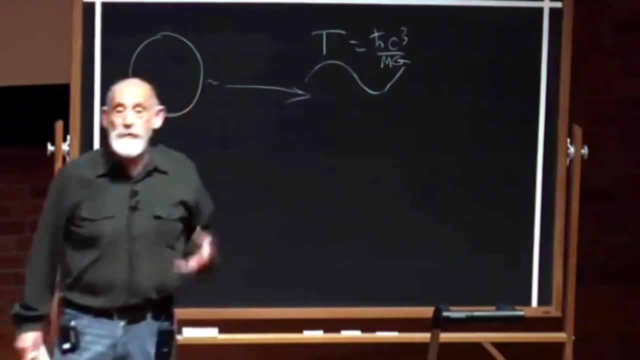 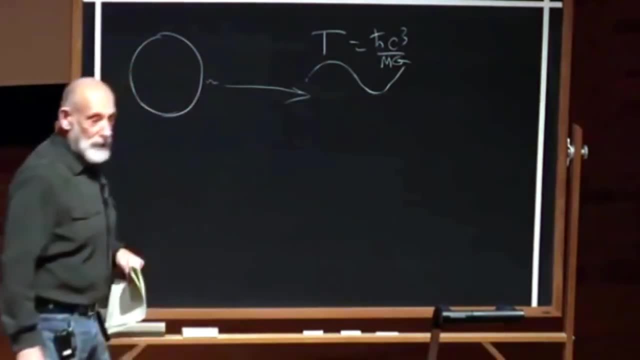 kinetic energy. That must mean when it started near the horizon, it had a lot more kinetic energy. And if it had more kinetic energy it effectively means that things were much hotter near the horizon. Bob falling in will not encounter a photon of this energy. This 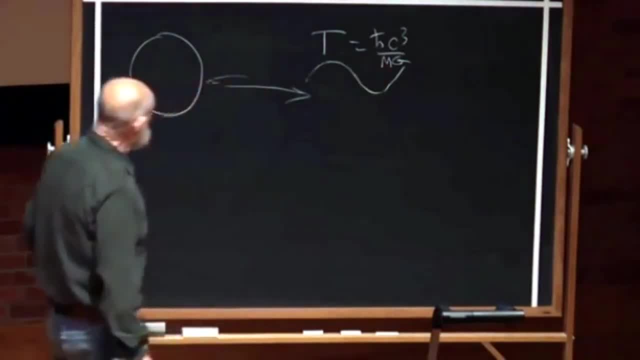 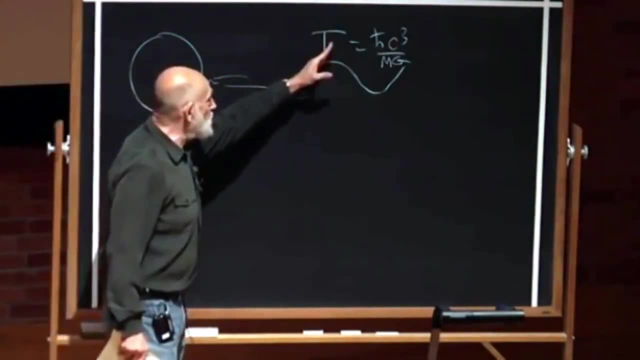 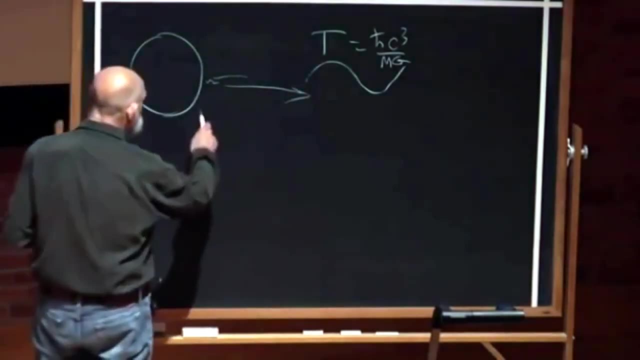 is very low because of the mass in the denominator. here He will encounter a photon of much shorter wavelength, much higher energy, just because if it got to be of this energy, by the time it got out it must have been much hotter. The energy of a photon, or let's just call it the effective temperature, the effective 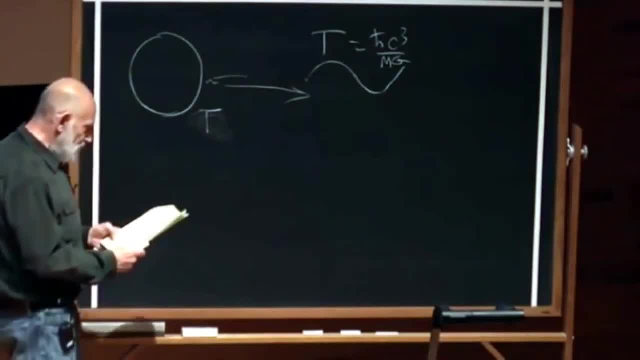 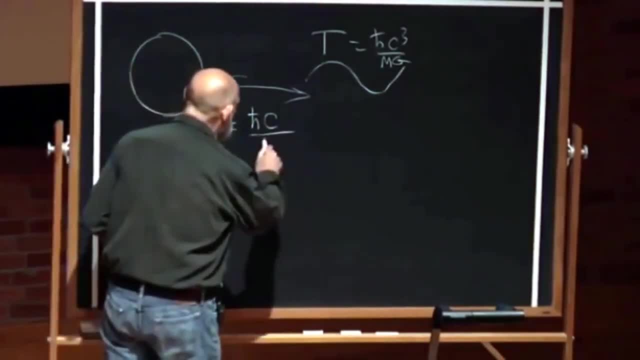 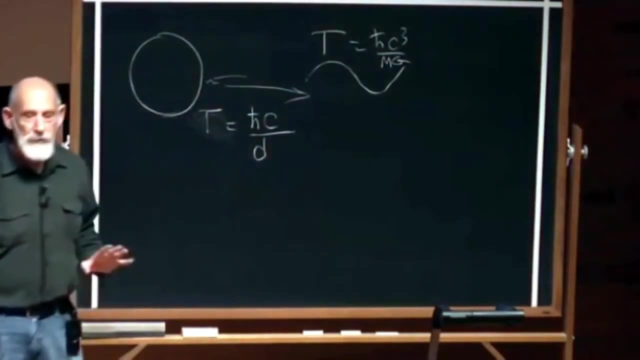 temperature at a distance d from the horizon, little d. that temperature is h bar c. that's not the important thing. divided by d, The implication is that as you go closer and closer to the horizon, the temperature gets hotter and hotter and hotter. 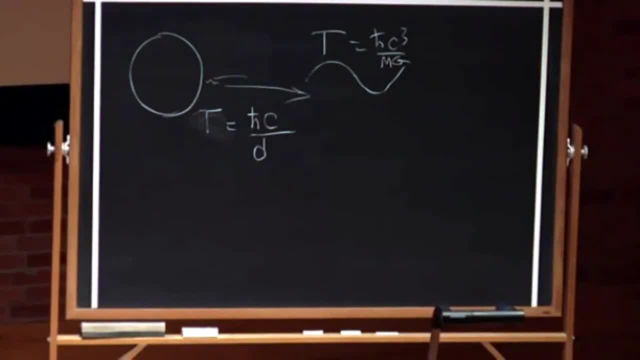 That could be bad news for Bob. Bob, who's going to jump in, will apparently encounter a huge temperature as he gets near the horizon. On the other hand, something very peculiar, because the equivalence principle tells us that when Bob falls through the horizon, discovers. 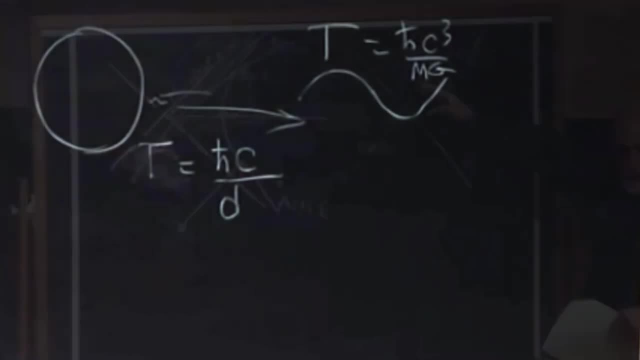 nothing special, just empty space near the horizon, And so we have a kind of conflict. We have a real conflict. I think, Well, I don't think it's a real conflict, I think there's an answer to it. I don't think it's a real conflict, I think there's an answer to it. 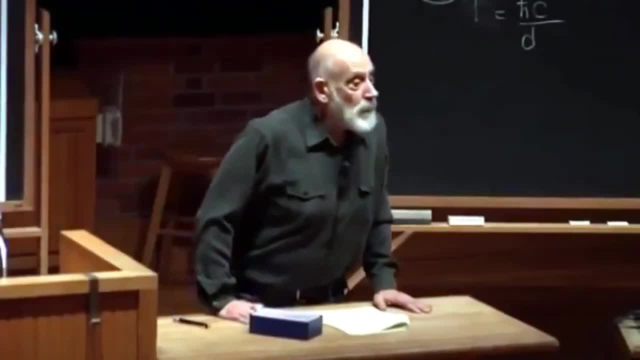 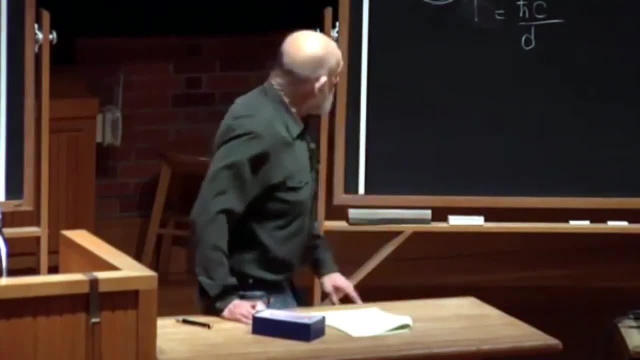 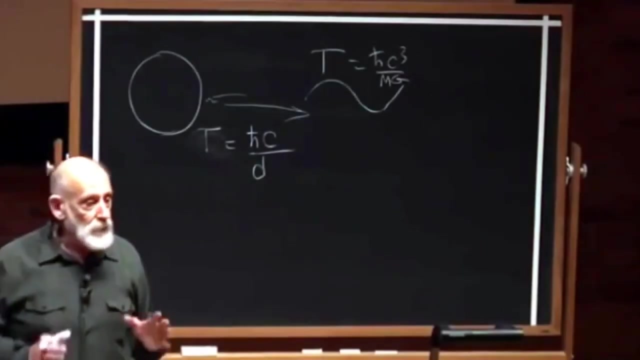 Let's just go back for a minute. What is Alice's description of this black hole? A pileup happens. The pileup carries lots of entropy. Apparently, it carries a lot of temperature. It's very hot near the horizon. Where did this all come from? It came from the assumption. 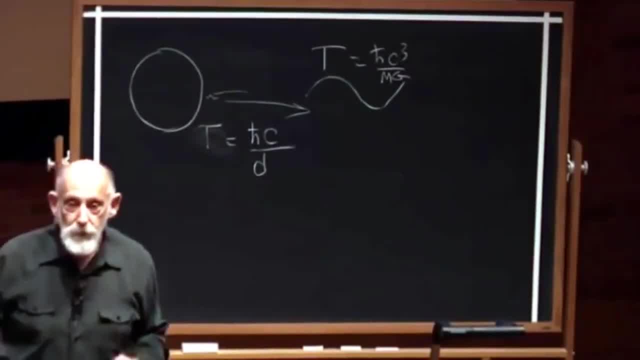 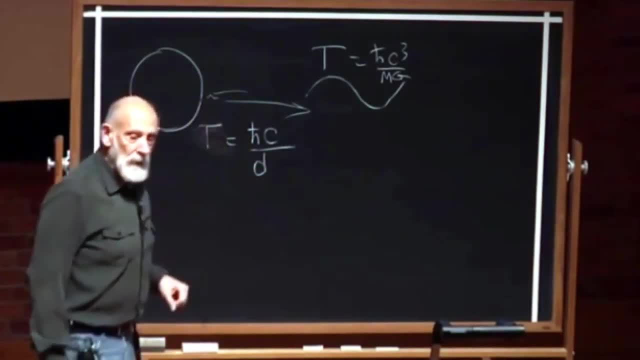 that information is conserved. How did we use information was conserved? Well, we said: anything that falls into the black hole gets piled up near the horizon, It doesn't get lost. So information conservation, on the one hand, tells us, or tells Alice, that there's a pileup. 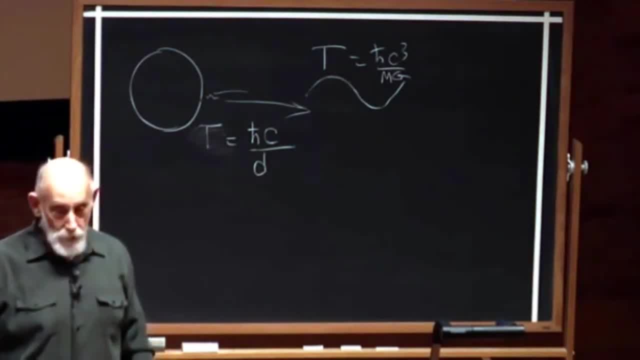 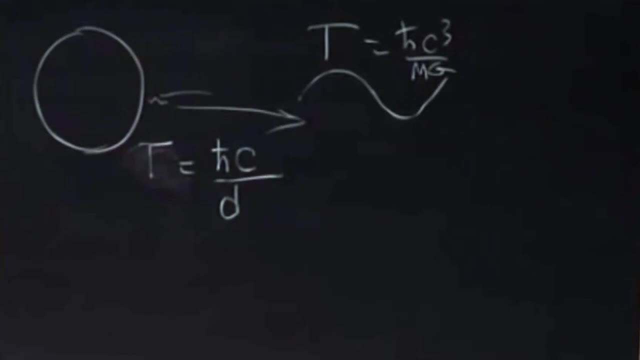 near the horizon. Bob, on the other hand, uses the equivalence principle and he says: Einstein tells me that a gravitational field is nothing but a field of acceleration, and under those circumstances I should discover nothing special when I pass the horizon. So 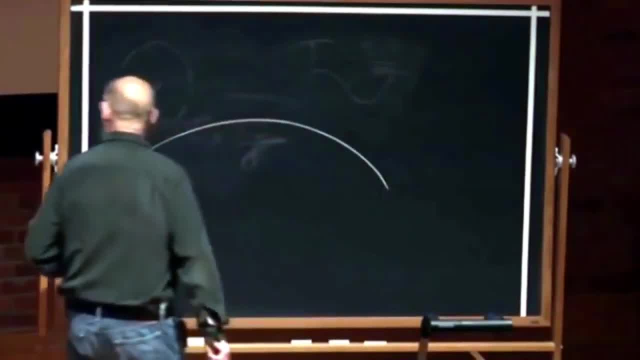 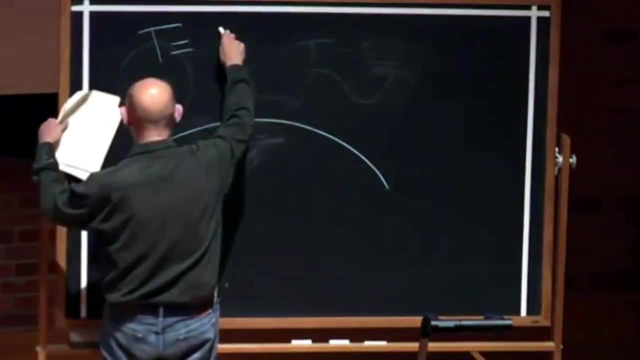 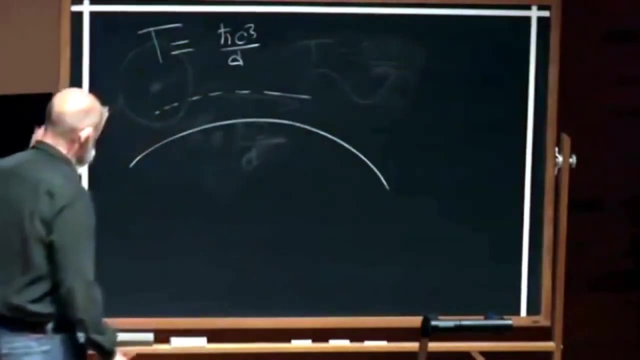 here's our horizon And using the formula, which I erased, that the temperature is equal to what did I say? it was H bar C, cubed over D, over the distance from the horizon. That's the distance from the horizon. Let me take the place, the place here, where the temperature is larger than 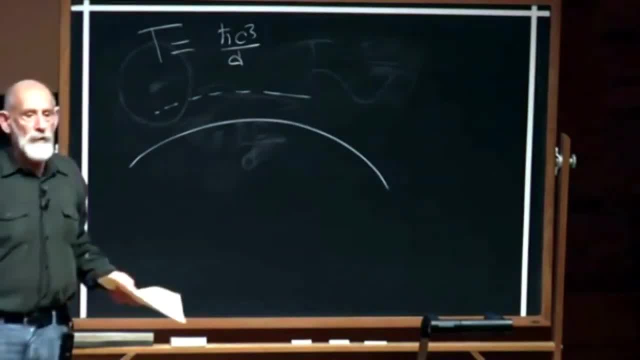 a certain temperature. What temperature? Oh, the temperature at which Bob will be scalded. Temperature at which Bob- Let's do something a little bit simpler. What temperature will be scalded? Oh, the temperature at which Bob will be scalded. Let's do something a little. 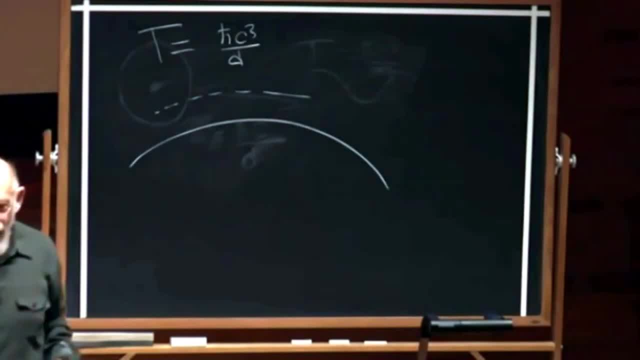 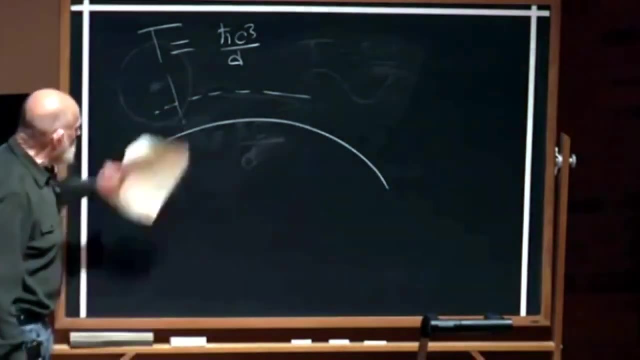 simpler. Instead of Bob, let's just drop an atom in According to this picture. if the atom gets close enough to the horizon, it runs into a place where the temperature is hot enough to ionize it. So an atom falling in according to this picture will get ionized. 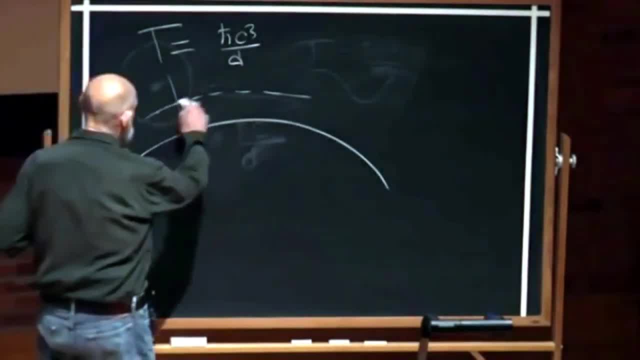 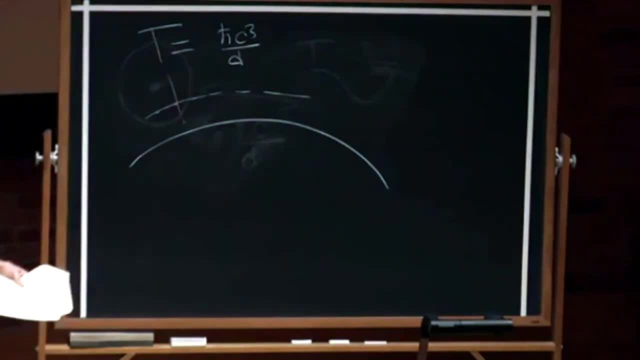 at a certain distance from the horizon. That distance is the temperature where the black hole or where this formula becomes what? 13.5 degrees Celsius, 13.5 electronvolts or whatever it happens to be the ionization energy. 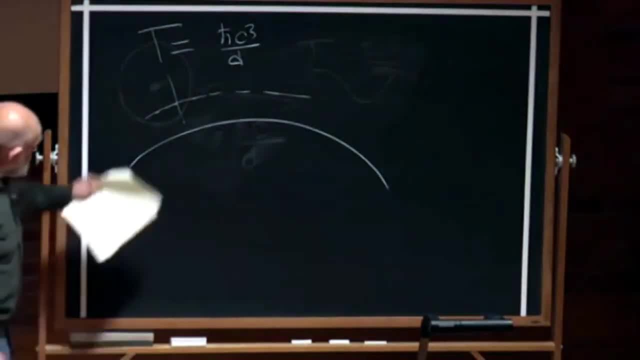 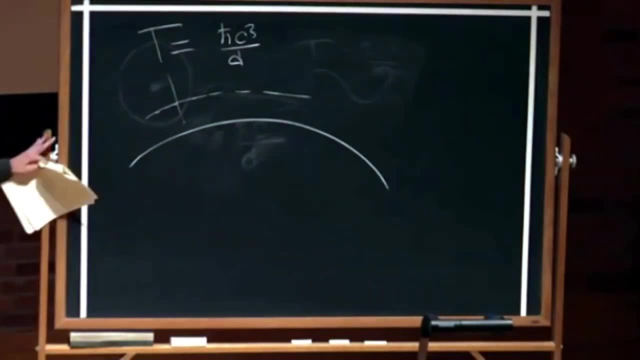 Okay. On the other hand, the other picture says that the atom just sails through. Let's do an experiment. Let's do an experiment of the following kind: Charlie- let's see Alice is here and she's watching all of this. Charlie is going to illuminate the atom with 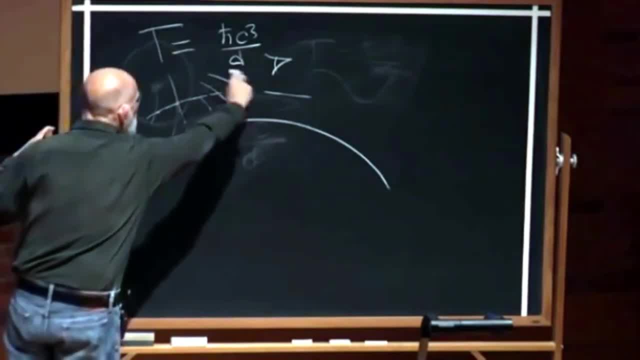 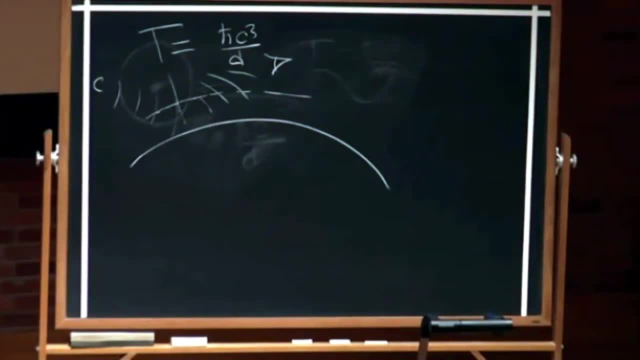 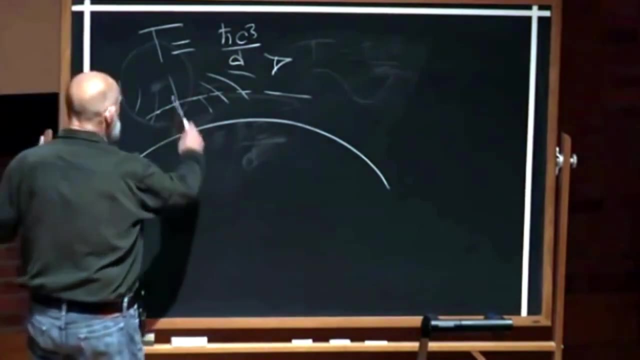 radiation that will bounce off so that Alice can see what's going on. I mean, what's going on? This is how you see things, This is how you find things out. You illuminate the system with, let's say, photons or with radiation and take a look and see what's going on. Question: 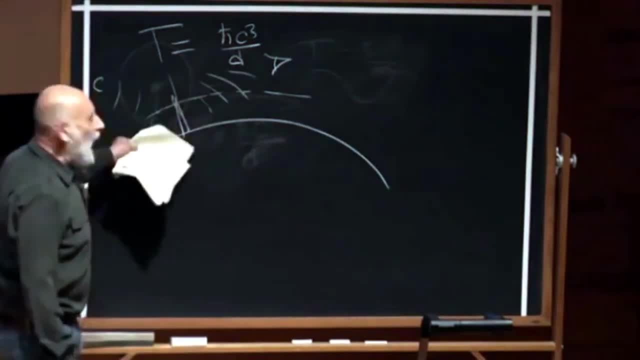 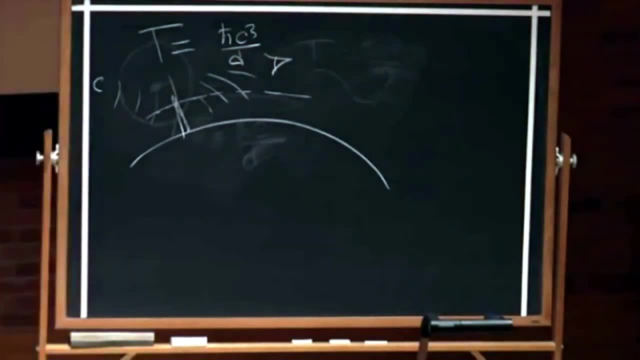 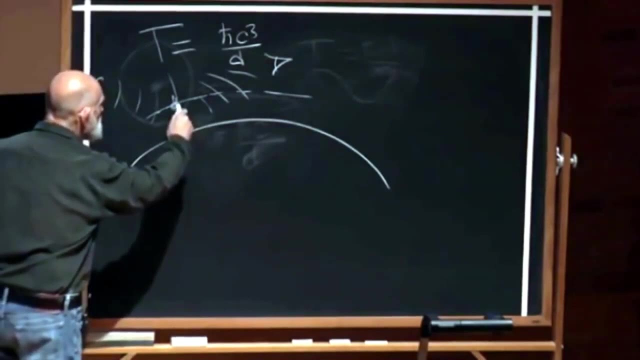 will Charlie's radiation come back to Alice and say the atom was ionized, or will it say that the ion was un-atomized? Okay, so let's see if we can analyze it In order for these photons to see what's going on in this small distance d here the photons have to have. 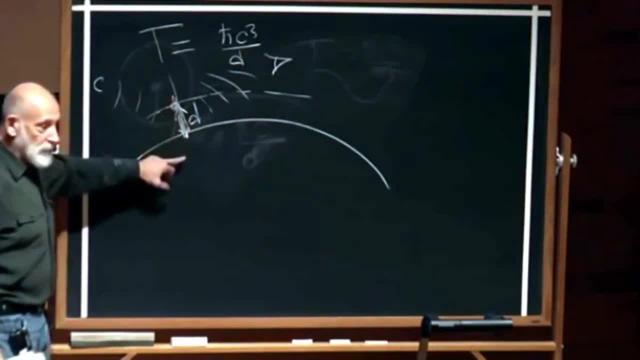 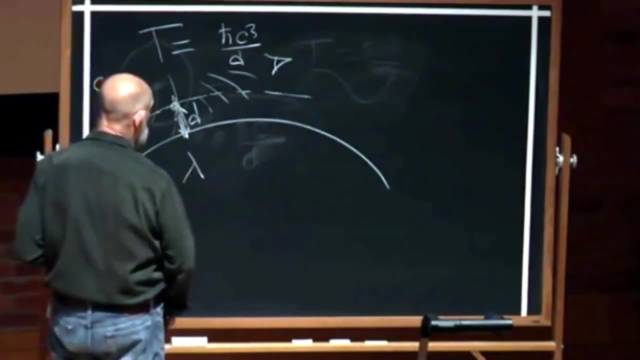 a small enough wavelength that they can resolve this distance. You can't see something of a given size with photons of longer wavelength, So the photons have to have a wavelength d or smaller. Lambda of Charlie's photons has to be d or smaller, So the photons have to 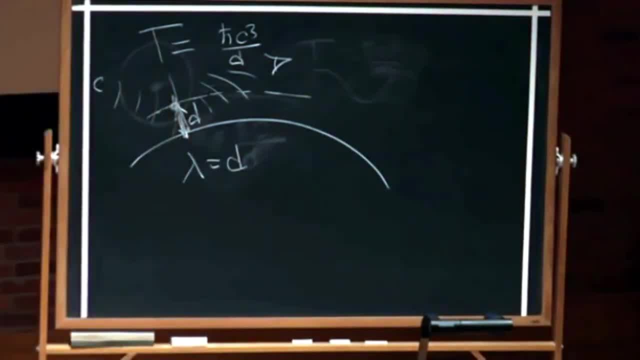 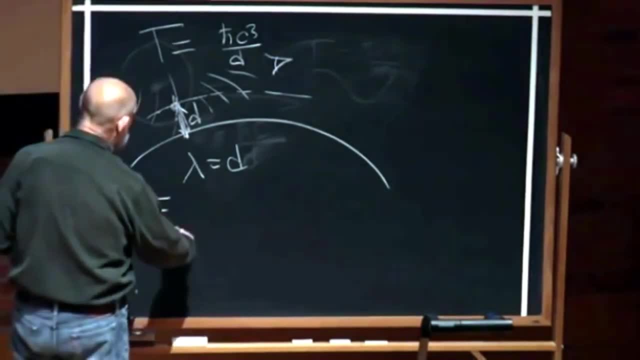 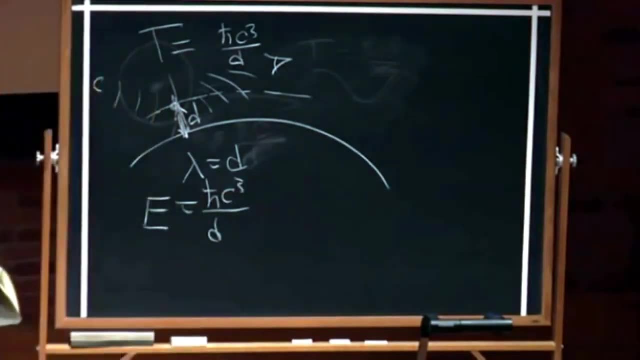 be d or smaller. From that we can compute what the energy of the photons is. The energy of these photons will be perhaps no surprise. the energy of those photons will be h bar c cubed over d. Did I get that right, Sorry? h bar c over d. The energy of the photons. 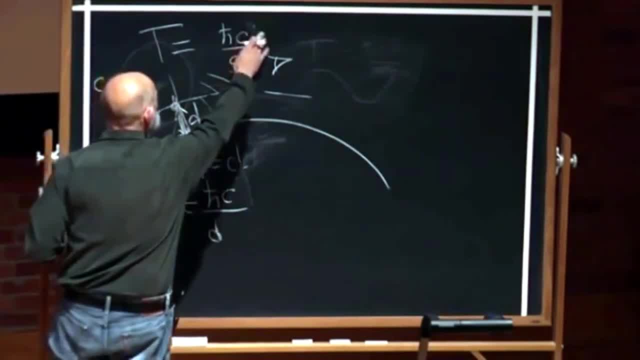 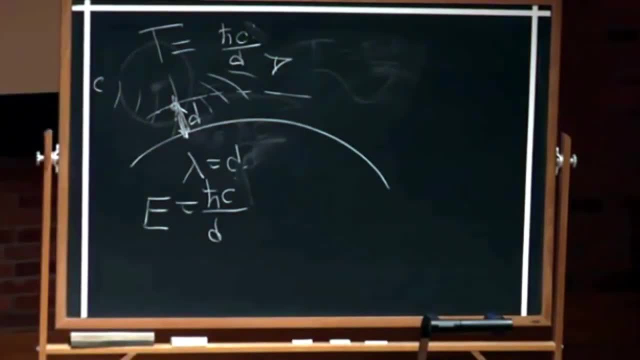 is h bar c. Is this right? This can't be right. Let's see, Let's see, Let's see Same thing. So this is with the first photon. So by that we can compute the amount of energy that Charlie. 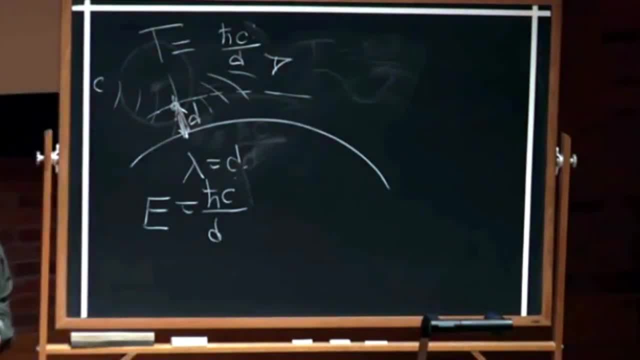 has to light on this system In the attempt to find out whether the atom was ionized. this is the quantum of the second photon, the quantum mechanism of the second photon. Alright, so here then is the energy of the photons that Charlie has to shine on this. 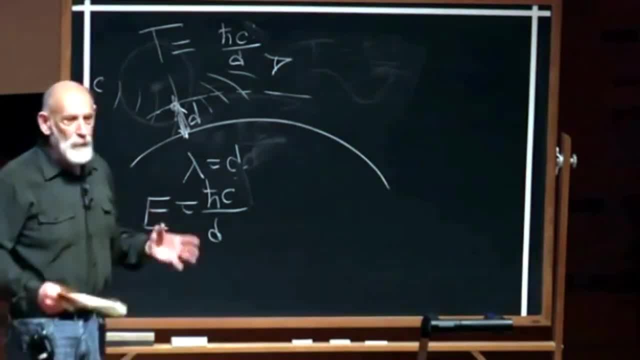 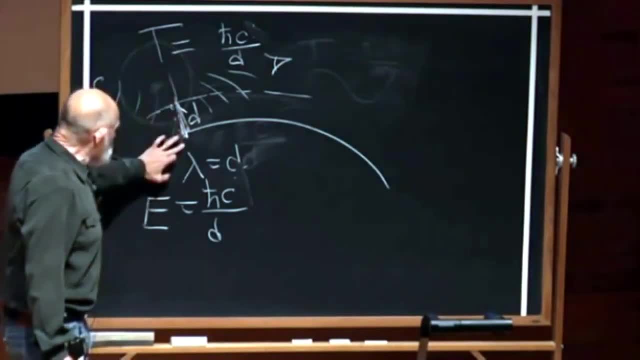 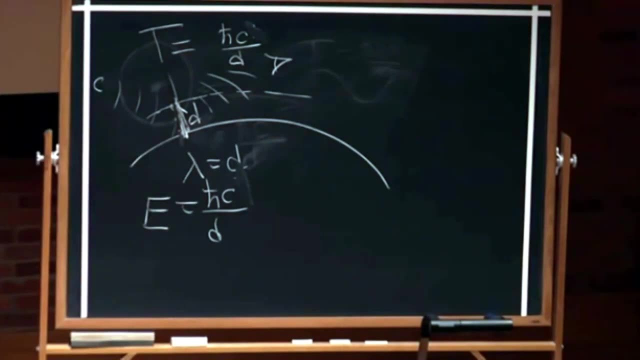 system. What's the problem? The problem is that these photons that Charlie uses to illuminate- back to what I originally started with, the experiment to try to see that the particle fell through without being ionized- will itself ionize the atom. This is a very, very general pattern. 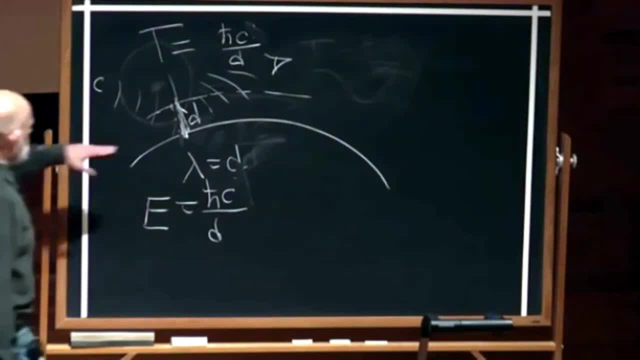 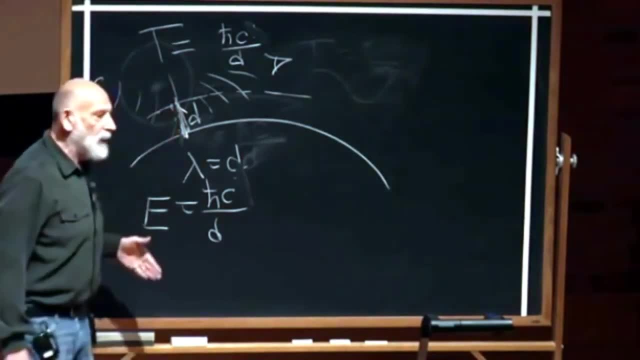 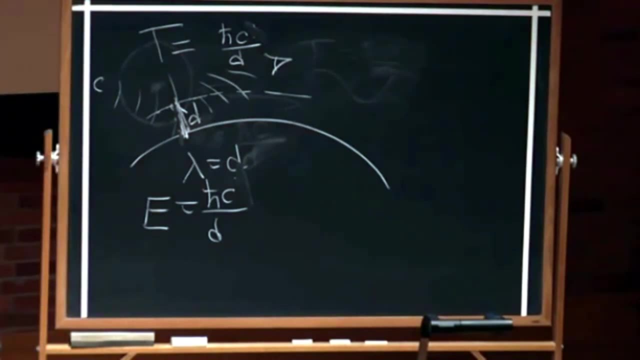 Any attempt to try to discover whether there is a pileup over here by shining light or anything else on the system to see what's going on will produce exactly the effect that the experiment was designed to show didn't happen. For example, when Bob falls through, Alice may want to find out whether he gets killed. 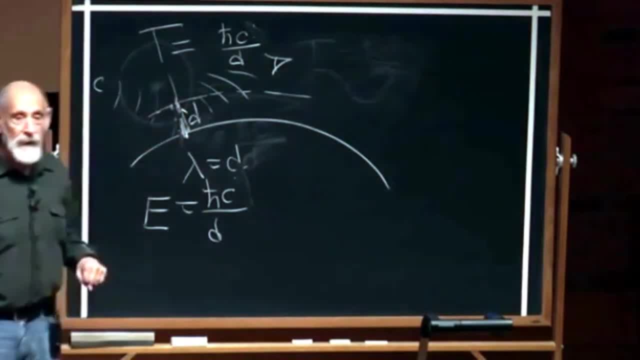 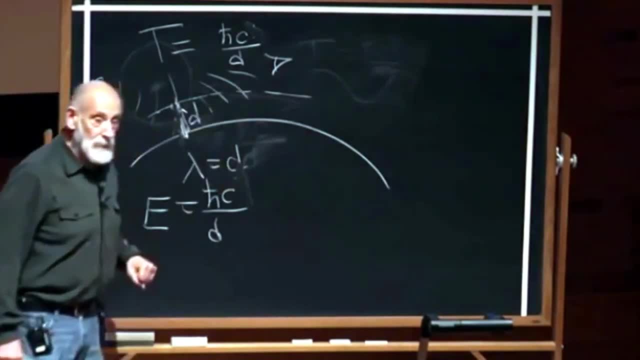 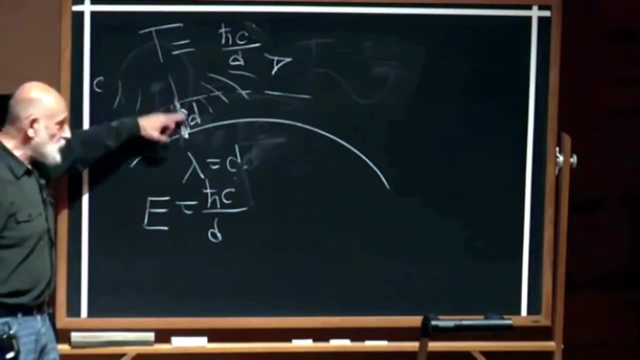 or roasted or fried or whatever it is at the horizon here. The only way she can find out is for Charlie to illuminate Bob with radiation and send it out to him. The answer will be that the radiation that Charlie has to use to see whether Bob was 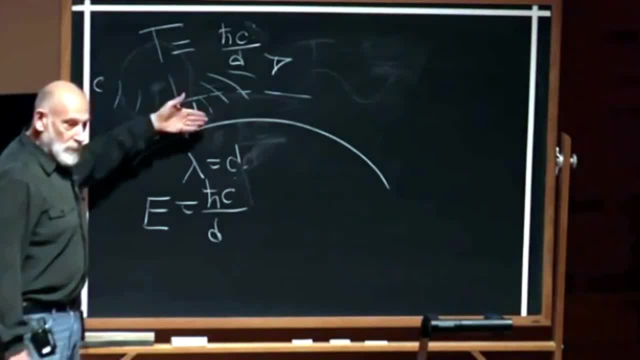 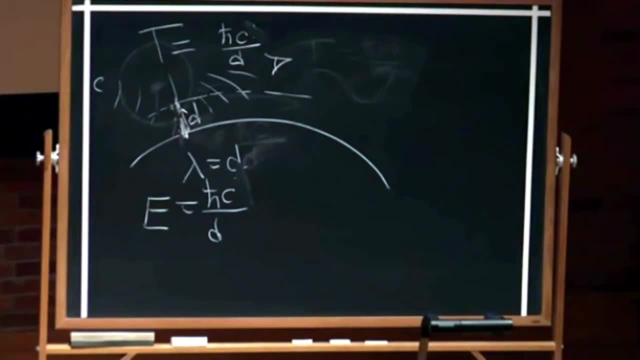 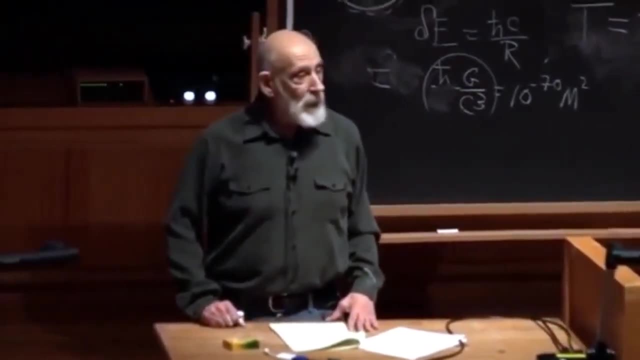 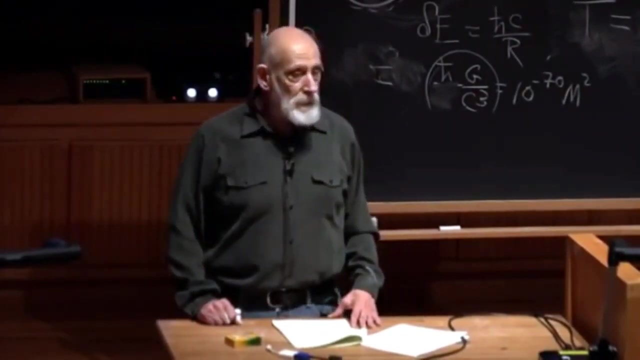 fried will have an energy hot enough to fry Bob. So I'm going to stop around here and tell you that, as far as we can tell, all evidence is that both descriptions are consistent, But they're complementary- Complementary in the same sense that the wave particle theory of light is complementary. 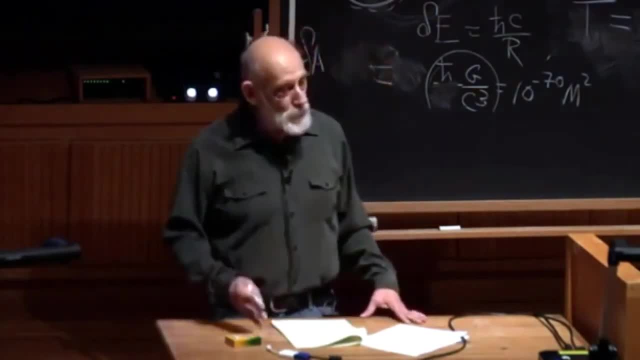 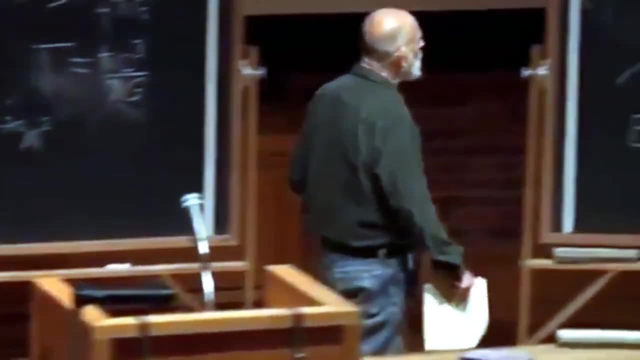 Complementary in the same sense that you can describe an electron by a position or a velocity, Not both. What we're learning is you should not try to think of a description of this black hole simultaneously from the point of view of Alice and Bob. 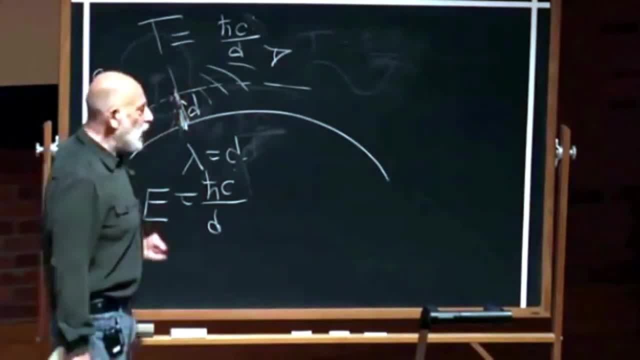 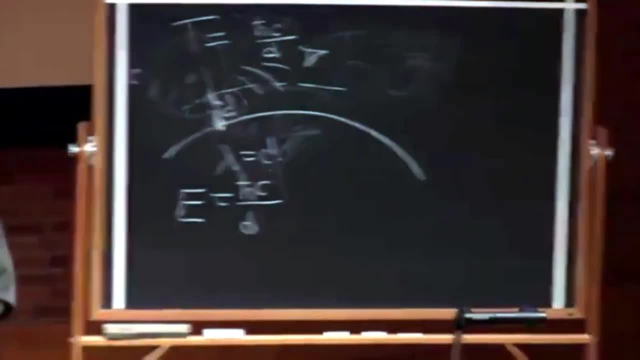 If you try that, you will run into trouble One or the other. Either you do Or you do not. try to find out if Bob was roasted. If you don't try to find out, Bob will fall through with no trouble. But Alice will never know. 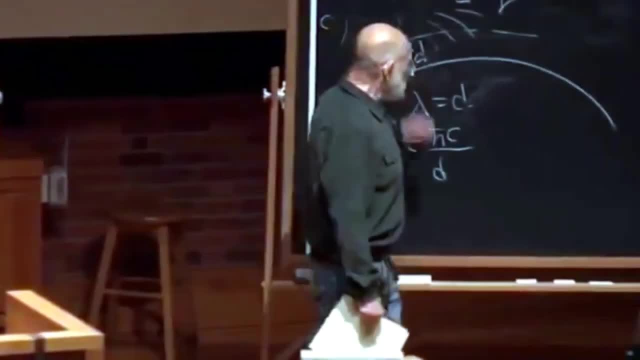 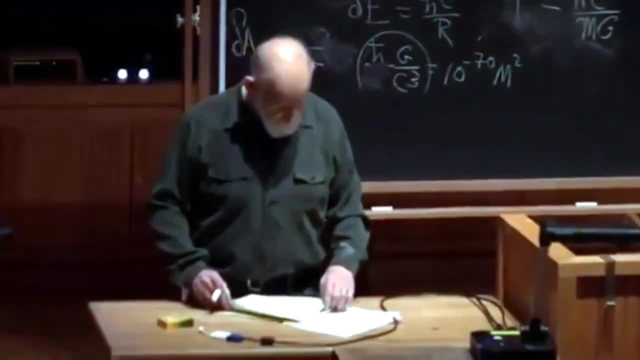 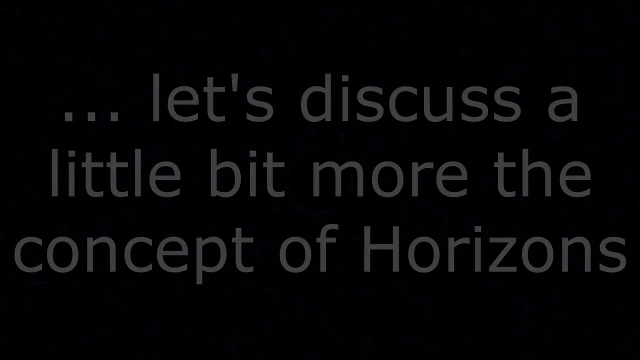 If Alice does try to find out, she will roast Bob. The evidence is that these two descriptions are not incompatible but complementary. I will stop at that point. In the field of astrophysics, an event horizon refers to a demarcation line beyond which. 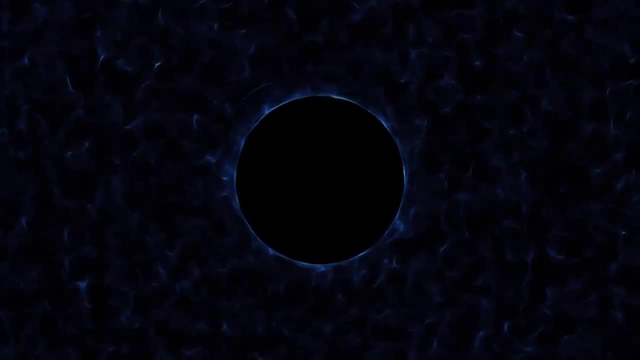 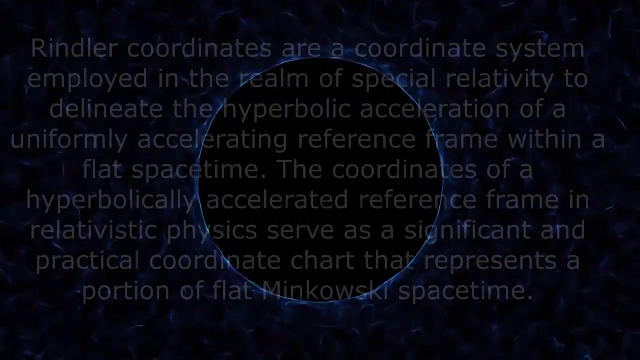 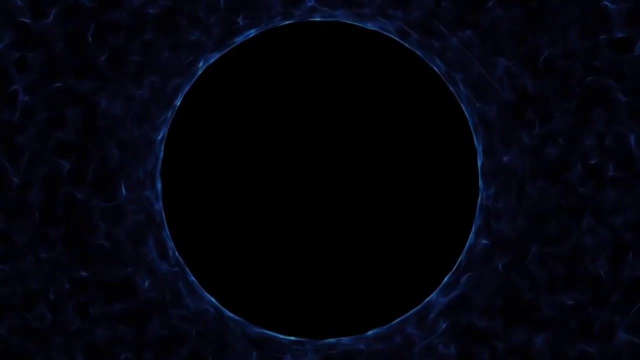 any occurrences are incapable of influencing an observer. The word was coined by Wolfgang Rindler in the 1950s. Some say that a Rindler horizon is an artefact of acceleration. Space continues behind it, And the Rindler horizon is both an event horizon. 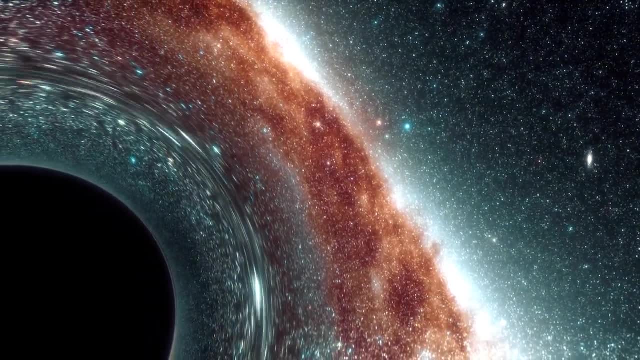 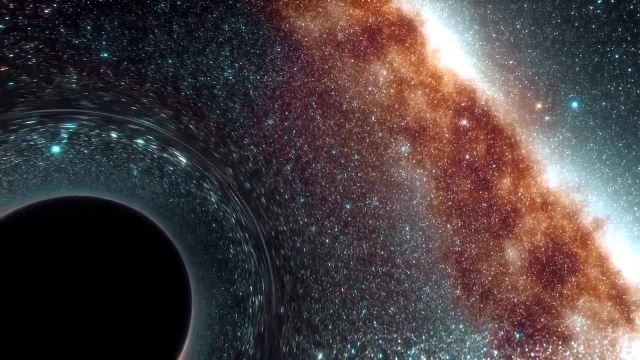 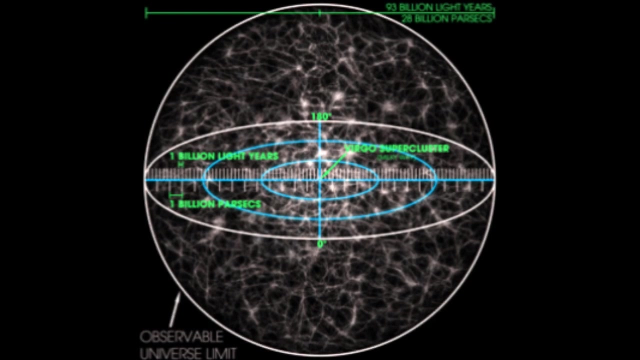 And a particle horizon, Nothing can be said to be behind it, like for any other horizon, because anybody who sees the horizon cannot observe anything behind it. The event horizon of the observable universe in cosmology refers to the maximum commoving distance from which light emitted at present can potentially reach the observer in the 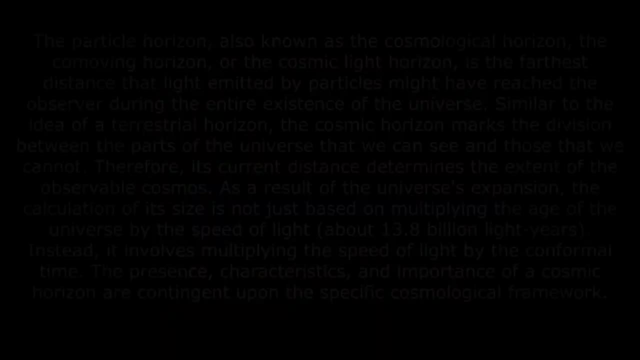 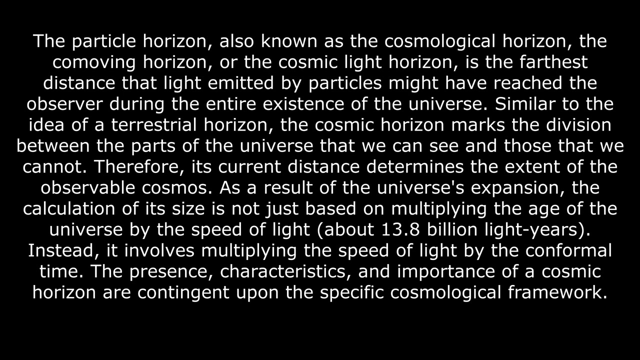 future. The concept of the particle horizon is distinct from this, As it denotes the maximum commoving distance from which light emitted at present can potentially reach the observer in the future. It is the maximum commoving distance from which light emitted in the past can reach. 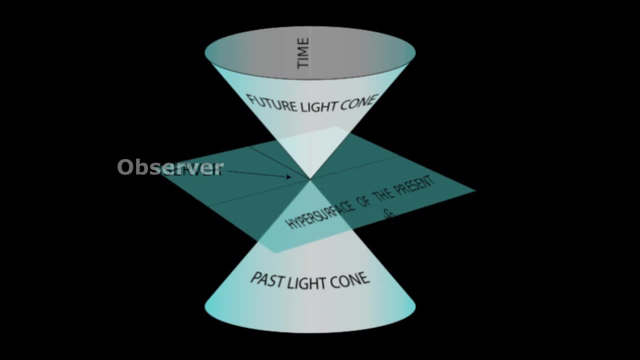 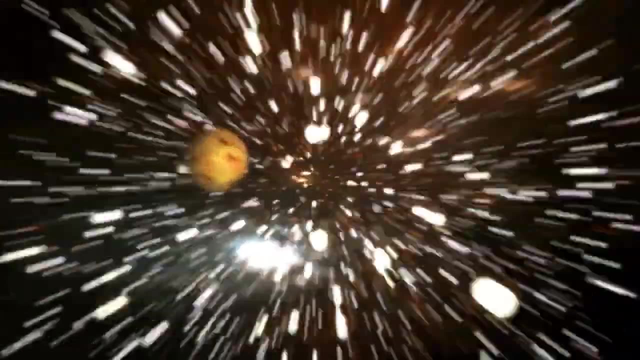 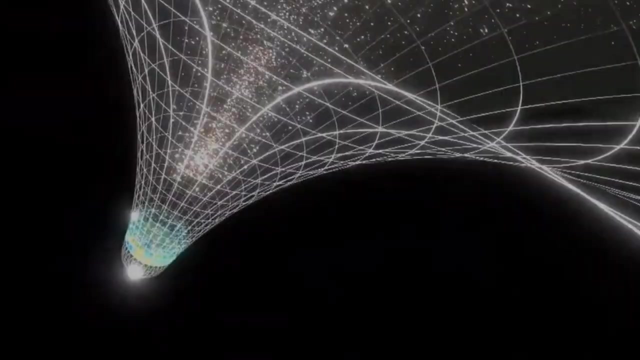 the observer at a specific time. Events occurring beyond that distance are beyond our observational grasp, as light released from those events at the beginning of the universe has not yet reached our location due to insufficient time. The temporal development of the particle horizon is contingent upon the characteristics of 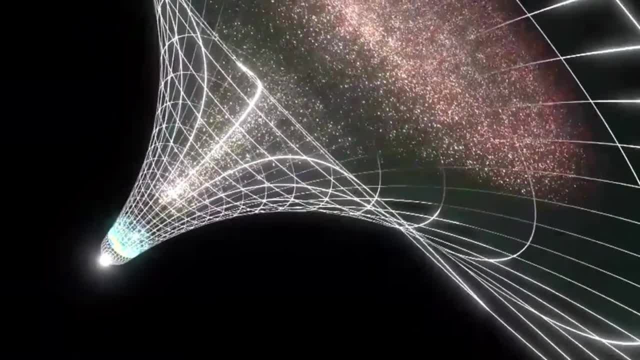 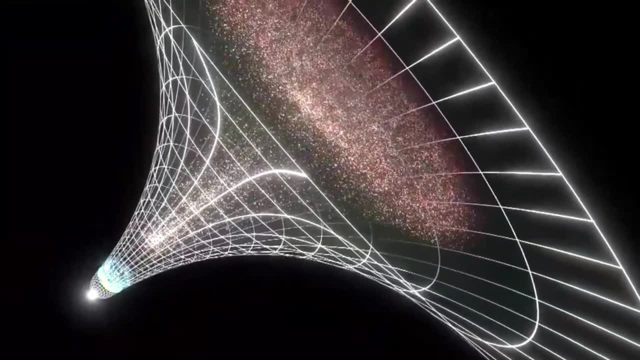 the universe's expansion. If the expansion exhibits specific attributes, then it is possible that the particle horizon will not be able to reach the observer at a specific time. As time continues to continue to move in the direction of light, certain sections of the universe will remain forever unobservable, regardless of the observer's patience in. 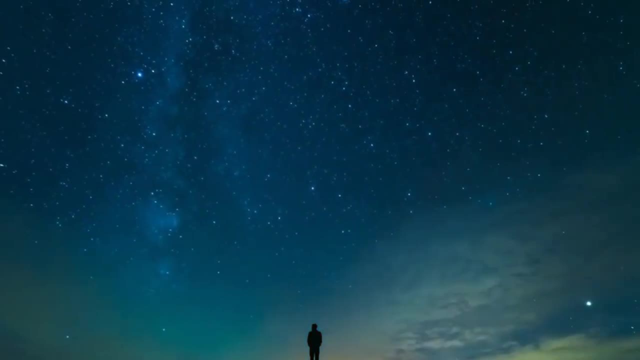 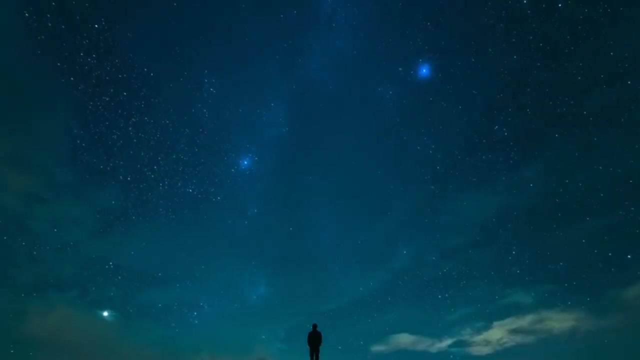 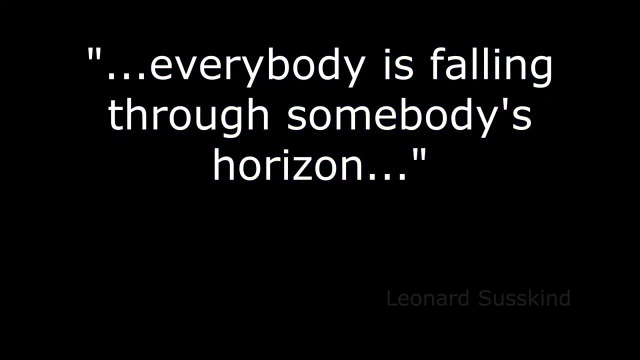 waiting for light from those areas to reach them. An event horizon is the barrier beyond which occurrences are permanently unobservable, serving as the ultimate limit of the particle horizon. Thank you for listening. Please feel free to leave a comment and share with us your ideas in the comments below. 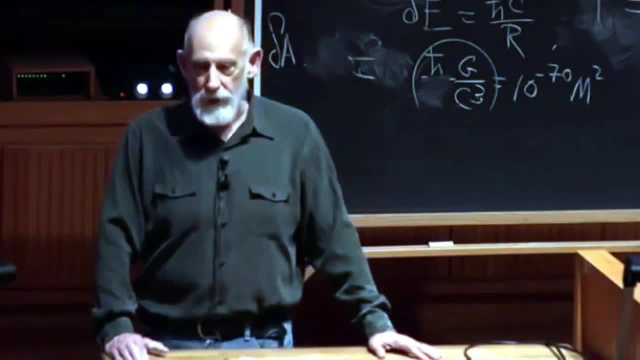 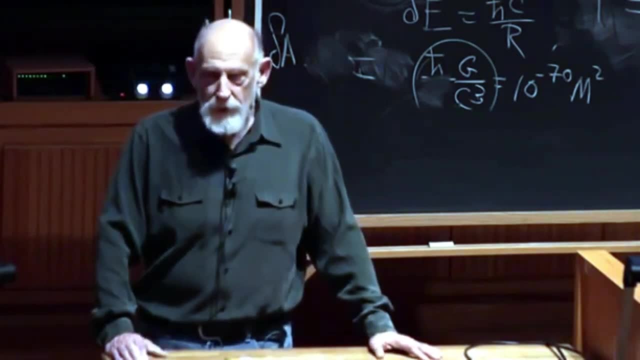 Thank you for your time. Do remember to leave your comments after the video and subscribe to our channel. Thank you for watching. In one description things fall in. In the other description they never get in. In Alice's description, which is appropriate to somebody who stays outside. 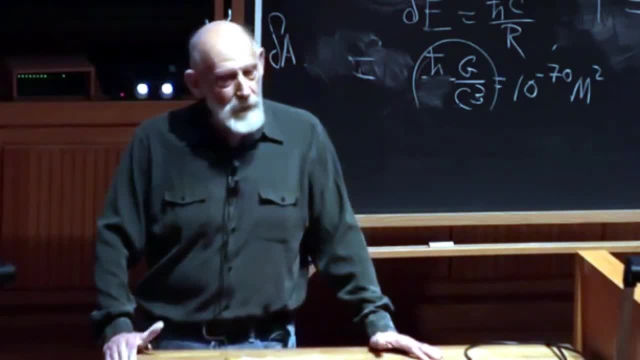 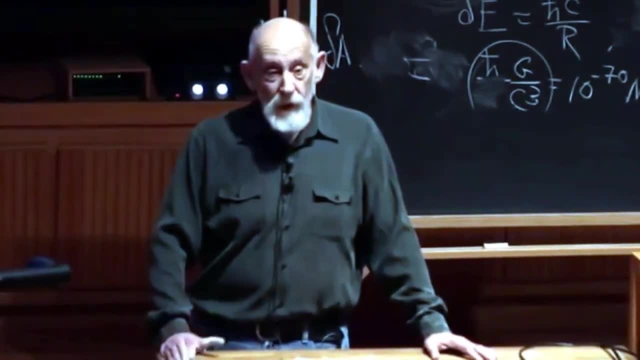 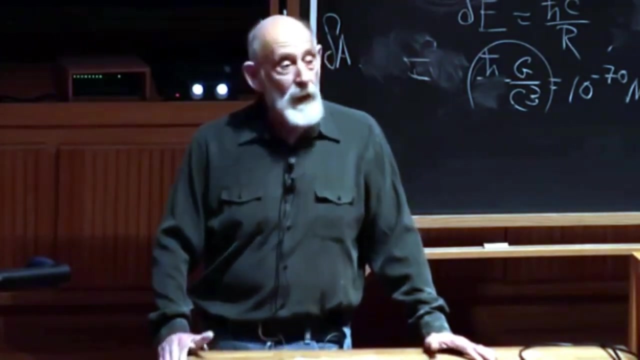 remember, somebody who falls in doesn't see this radiation. Somebody who falls in has a short amount of time before they're squashed to annihilation at the singularity. Somebody who stays outside sees the radiation. So we can ask what is Alice's description of things? 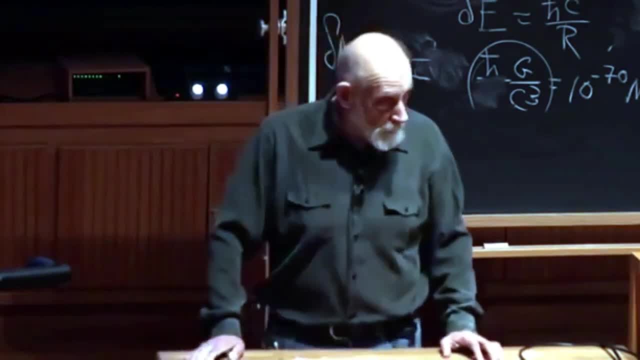 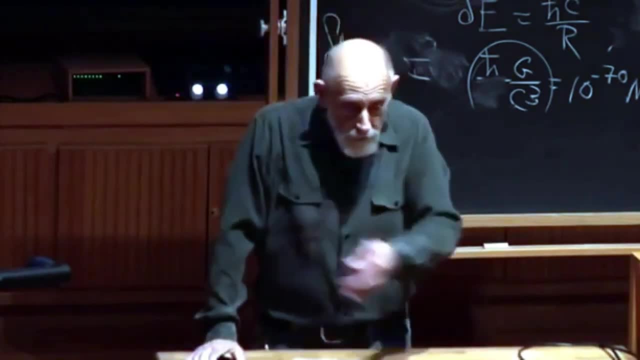 Alice says there's a pileup and all these degrees of freedom pile up at the horizon. they stick around there and gradually, sort of one by one, they boil off Bob, who fell into the black hole, destroyed at the horizon, at the singularity. 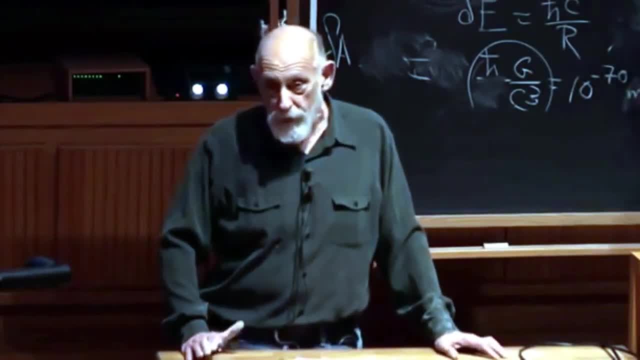 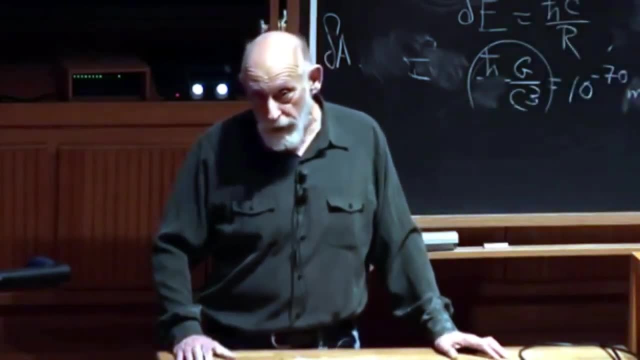 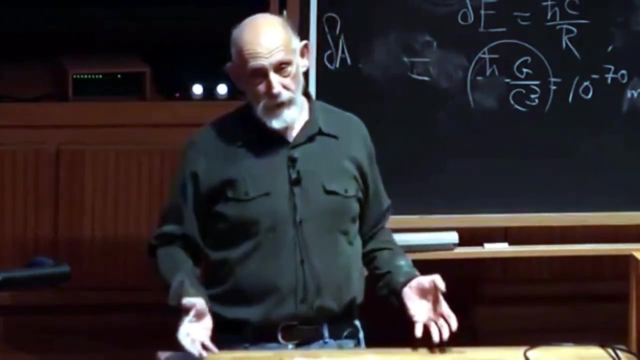 and simply wasn't around long enough to know whether the black hole evaporated. He's gone in a small fraction The amount of time for a solar-mass black hole that you know. the numbers here are a little bit deceptive. A solar-mass black hole is about a kilometer. 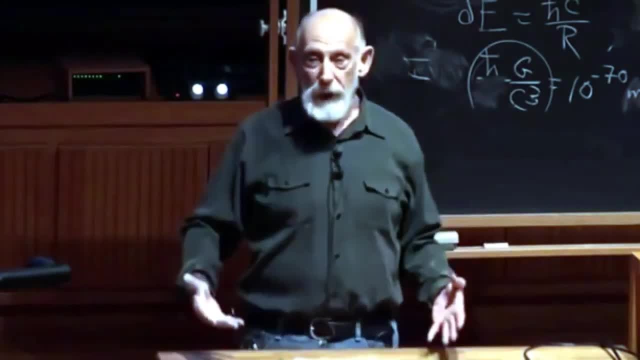 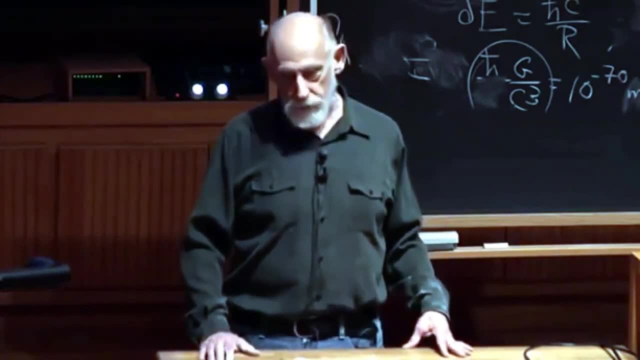 You might think that a meter's worth of human being could fall through a horizon a kilometer big. No, it turns out that the tidal forces at the horizon would be so strong that they would tear you apart. But that's not the important thing. 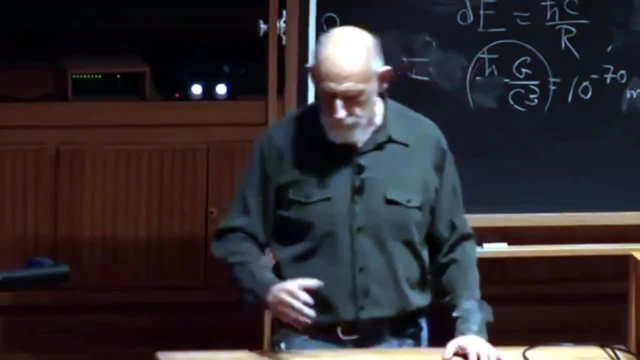 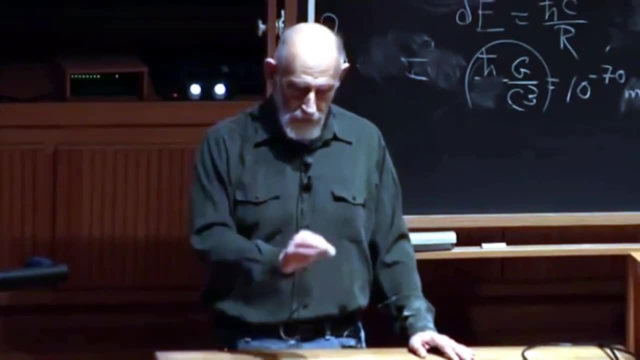 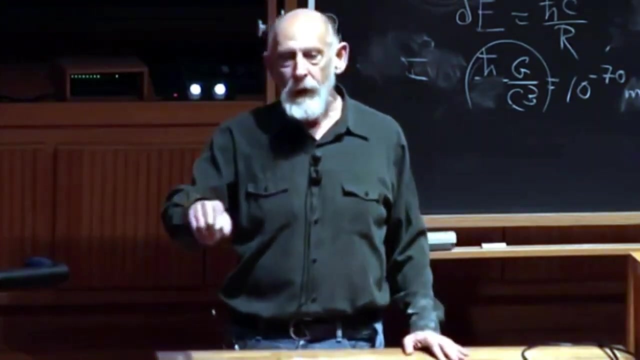 A much smaller thing could fall through. a bacterium could fall in. How long would the bacterium last? How long would the bacterium have before it fell and hit the singularity? And the answer is: approximately the light transit time across the black hole. 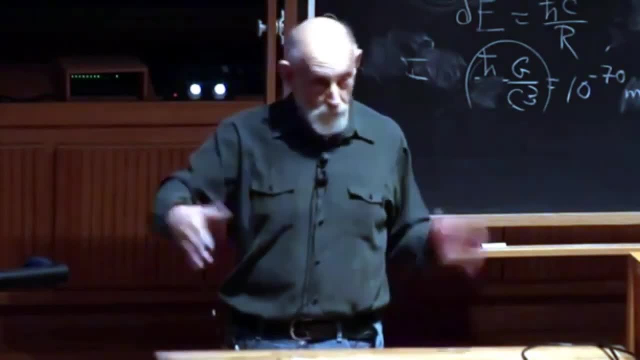 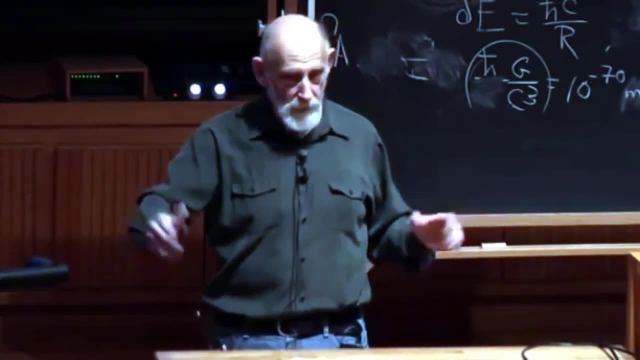 That would be about a millisecond, I think. I think it would be about a millisecond For one kilometer. anybody can do that fast in their head. One kilometer, I think it's about a millisecond. So that bacterium has about a millisecond. 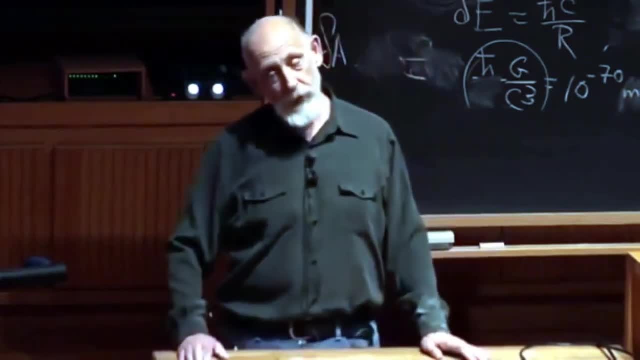 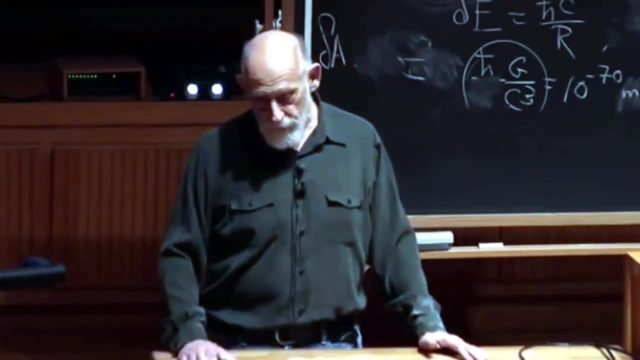 How long does it take the black hole to evaporate? Oh, just a tenth of a second. Oh, just a tenth of a second. It's about a tenth of a seventy-five years, or something like that. So the answer is that Bob has no experience of the evaporation. 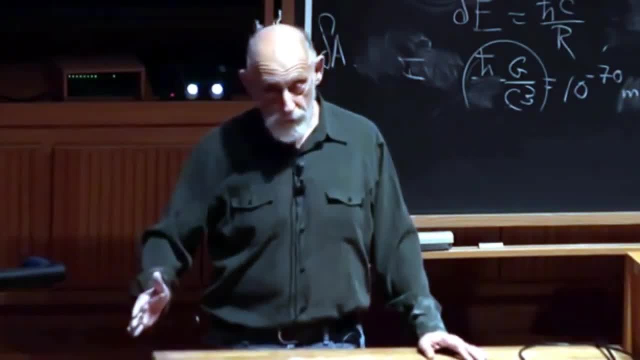 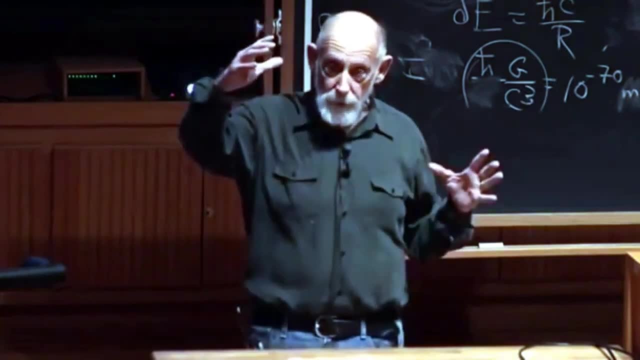 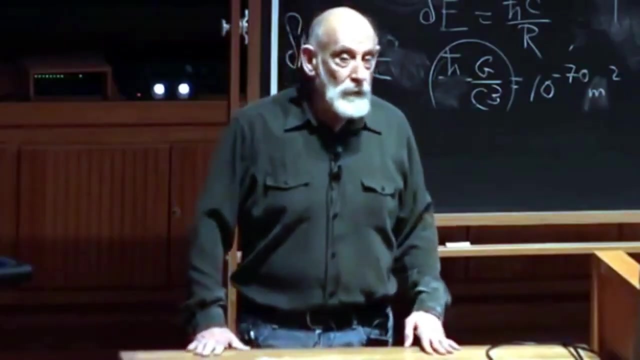 It's Alice whose story involves the evaporation of the black hole, And her story is that there's a pileup at the black hole and the pileup gradually evaporates off the surface of the black hole. So it's quite confusing, Of course, if it's a rotating black hole, which most black holes are. 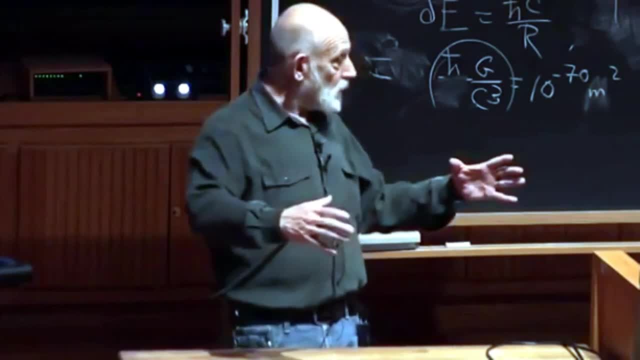 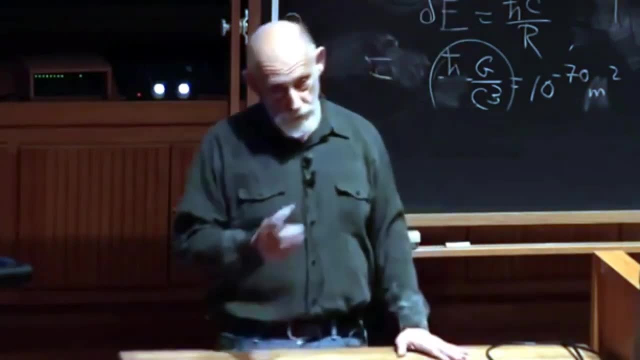 then it's a sort of oblate Oblate. do I have it right? Oblate is the broad one and prolate is the skinny one. Yeah, It's an oblate spheroid, which means a sort of ellipsoid. 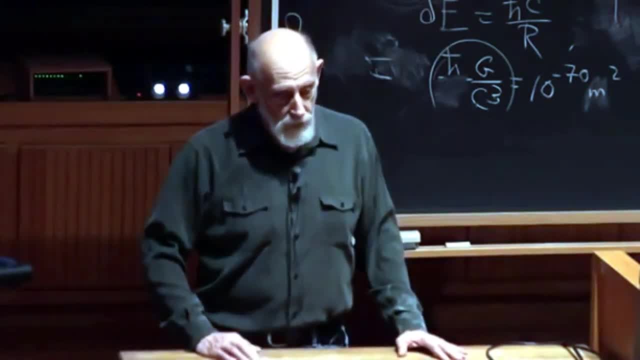 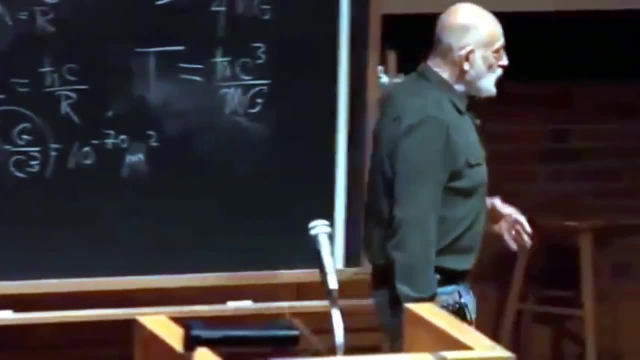 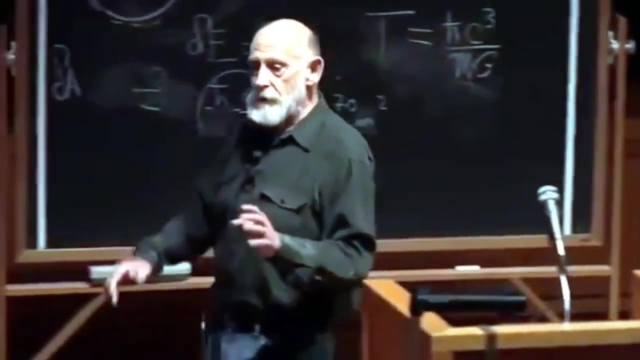 But if it's not rotating, it is spherical. Now one answer to it is: a black hole is a thermodynamic system. A black hole is a thermodynamic system and that means it's a system which will come to thermal equilibrium. When a system comes to thermal equilibrium, it becomes featureless. If a system is spherically, no forget whether it's spherically symmetric- If an idealized system, such as a water droplet in space or something like that, which is a thermodynamic system, is allowed to relax to thermal equilibrium. 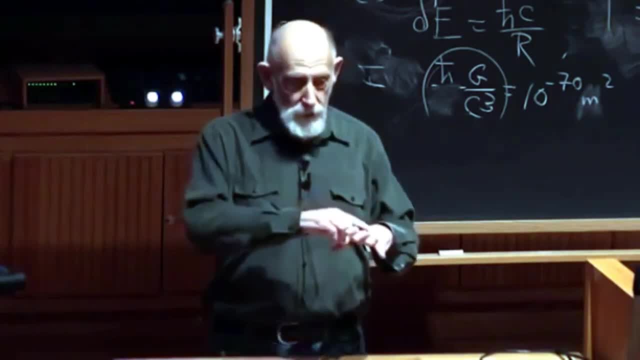 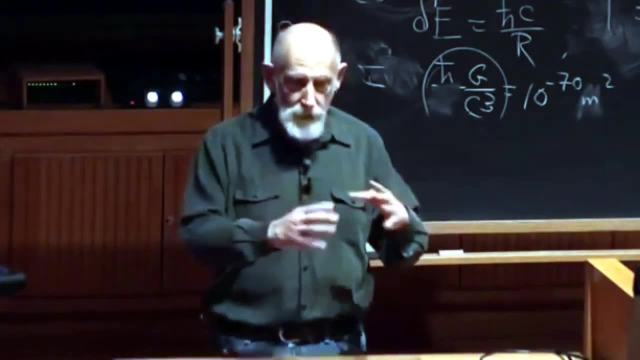 it will be perfectly round. One of the reasons is that the temperature has to be uniform everywheres across it- Temperature, pressure and so forth- so it will achieve a perfectly round behavior, and the black hole is also a thermodynamic system. 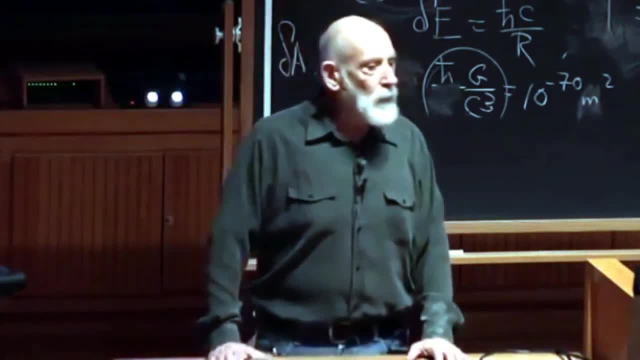 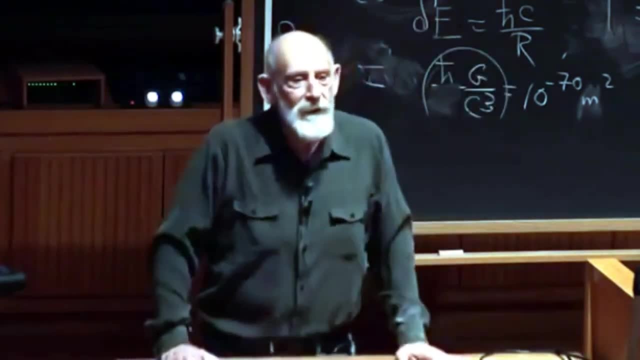 which comes to equilibrium. The words that John Wheeler used was a black hole, has no hair, which means it's sort of bald like my head and perfectly round Alice said. Alice has no use for it. She never heard of it. 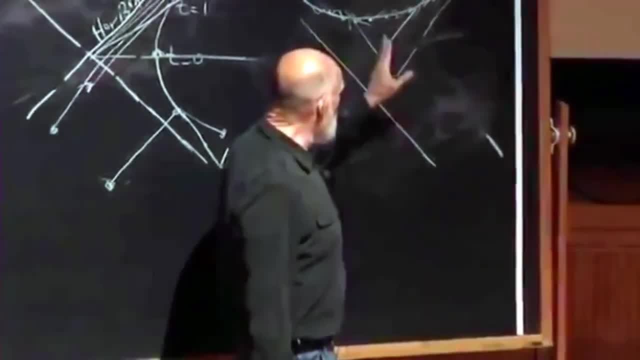 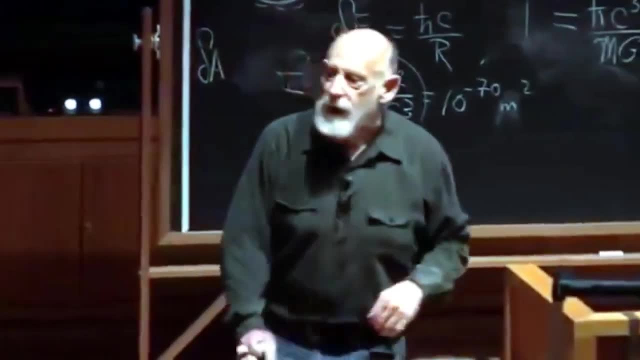 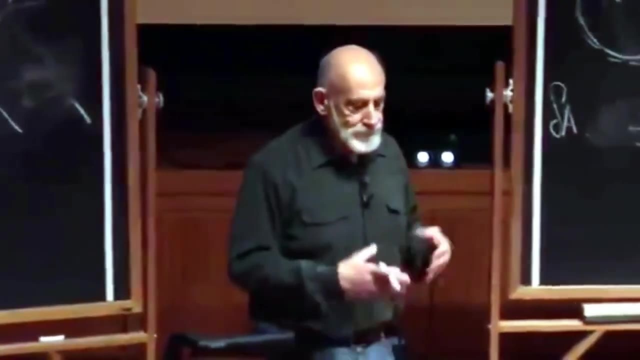 She said: the world ended over here. Bob, yes, and what does Bob say? It's just flat space, It's just a normal vacuum, normal empty space, except that it starts to get curved and distorted and deformed to the degree where it will become very harmful. 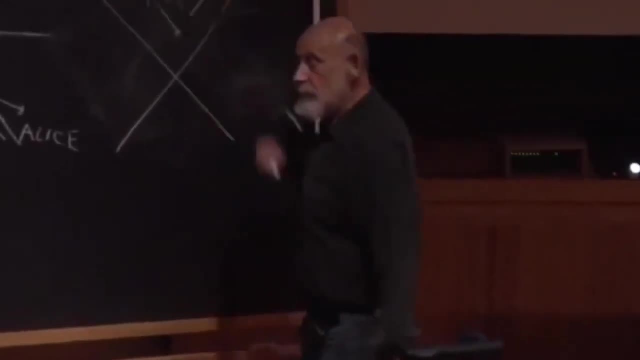 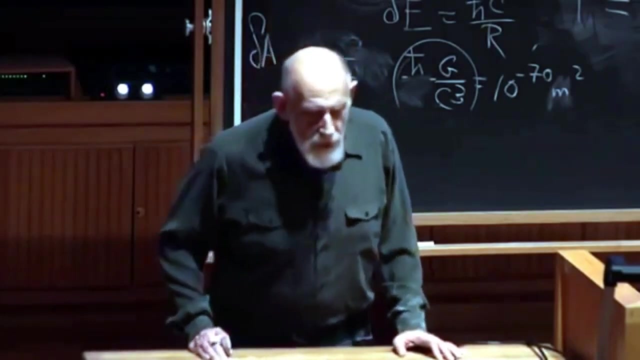 as he gets close to the singularity. As long as it's not too close to the singularity, it's just ordinary empty space. In some sense, the gravitational force is increasing, but it's increasing. in particular, the tidal force is increasing. 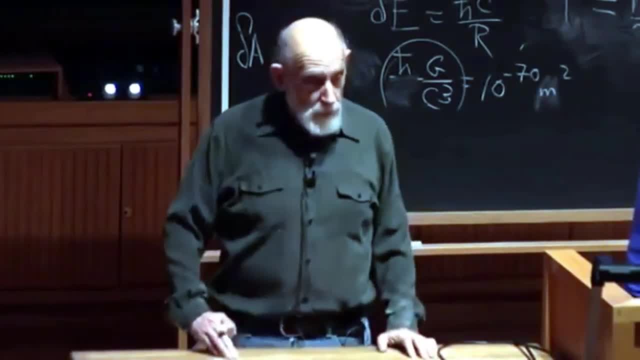 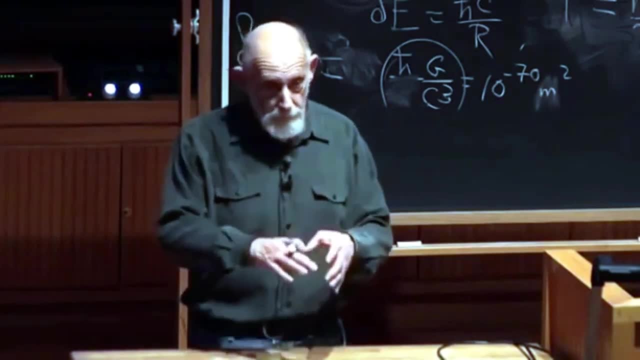 The tidal force is the thing that pulls you apart. The tidal force is increasing, but if we don't think about the tidal forces, if Bob is small enough that the tidal forces don't disrupt him, then he's just in free fall. In free fall, there is no gravitational field. 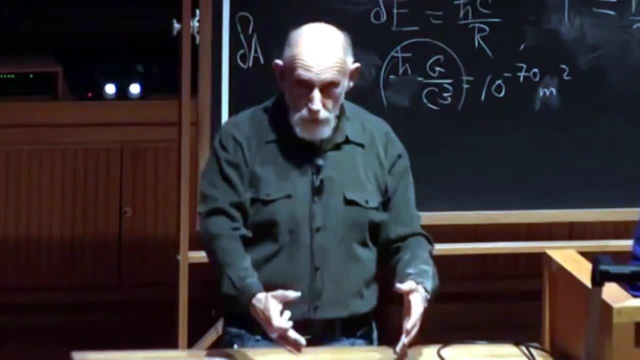 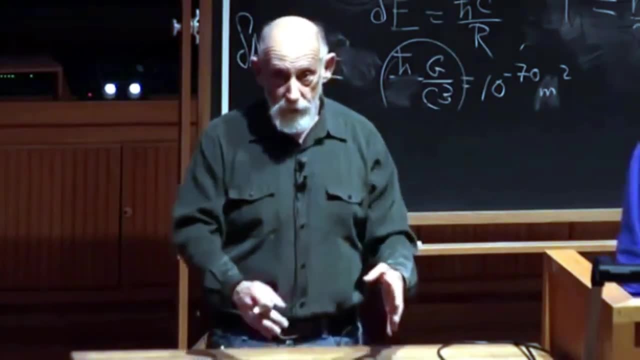 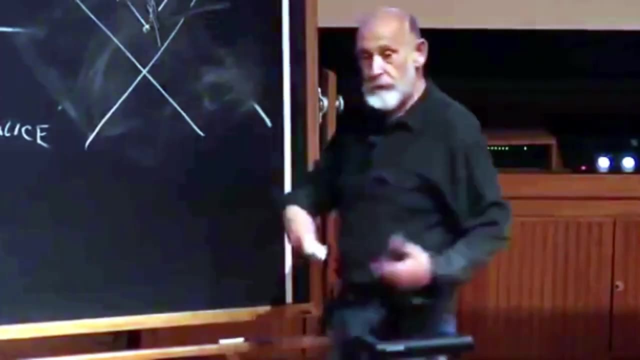 If you jump from the ceiling and fall down to the floor, you don't realize, with your eyes closed, of course. you don't realize that you're falling until you hit the floor. So Bob is in free fall. He says everything is perfectly okay. 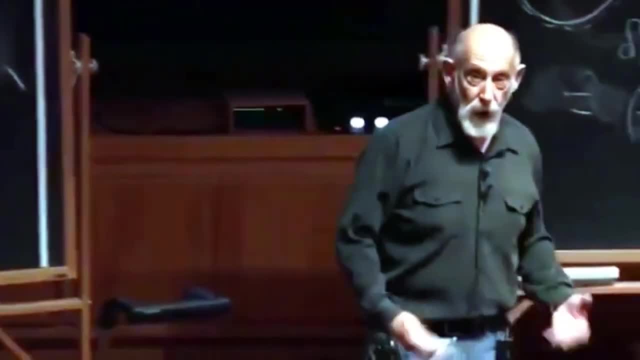 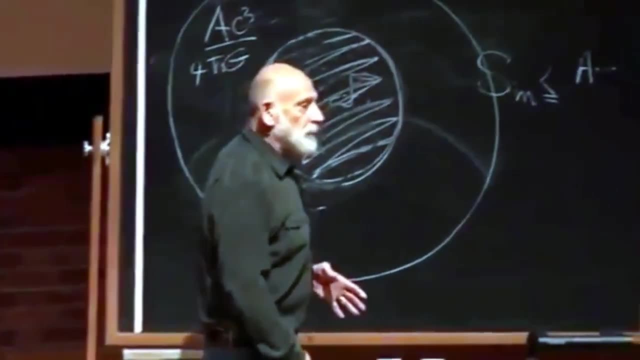 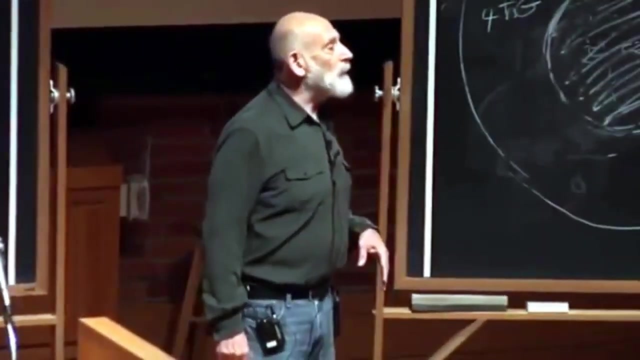 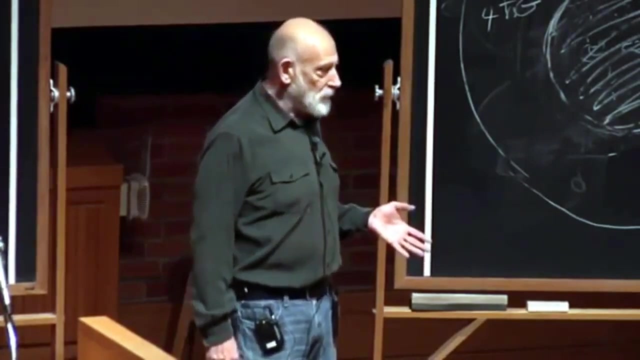 until he gets too close to where the geometry becomes highly deformed. What I would say is: this has implications for cosmology. Remember, in cosmology, everybody is falling through somebody's horizon. In cosmology, in desider space, Am I talking a language you are familiar with? 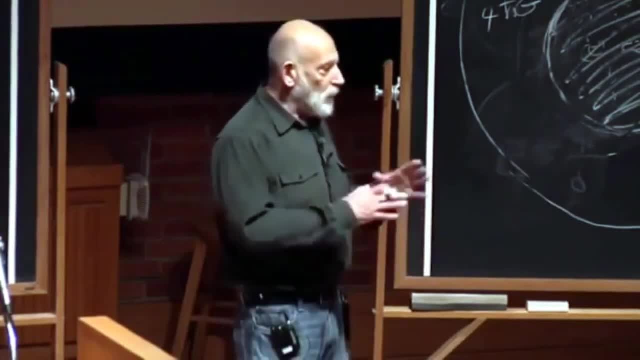 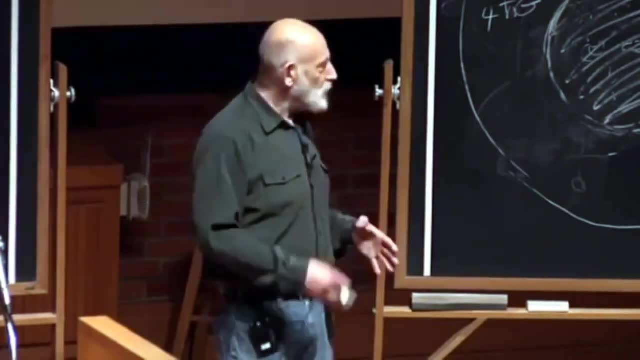 All right. In cosmology, everybody is falling through somebody else's horizon, And so just the fact that we don't get destroyed every fraction of a second means that horizons are smooth. You know you're asking a question which I don't know the answer to. 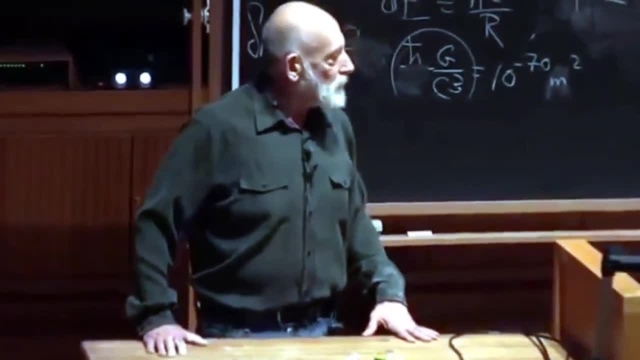 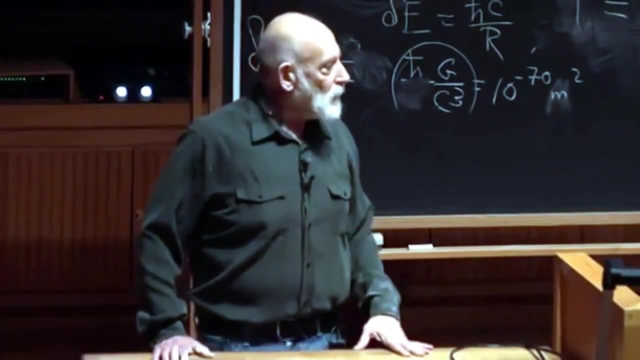 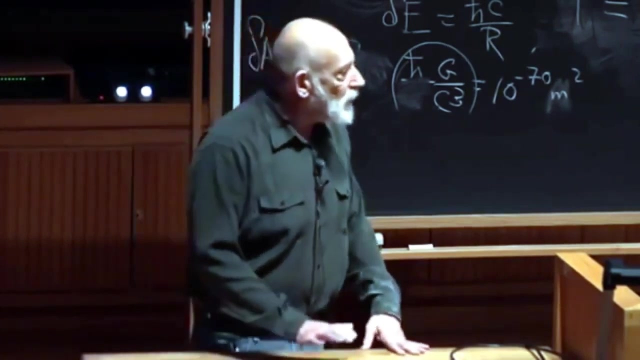 How do you make empirical science out of any of these questions? This issue has been around since 1974.. It has invaded physics to the point where I would say the majority of papers in theoretical physics, including condensed matter physics these days is using the mathematics of horizons and so forth. 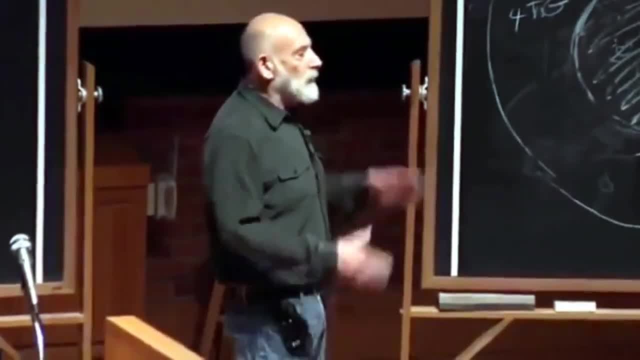 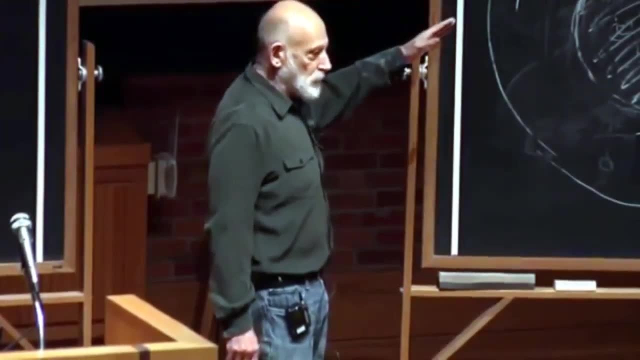 But it really is troubling. All right, let me just put it bluntly: It's very, very troubling that we've entered such a range of parameters that it seems absolutely out of the question to do experiments, Even if I told you that you could do the experiment. 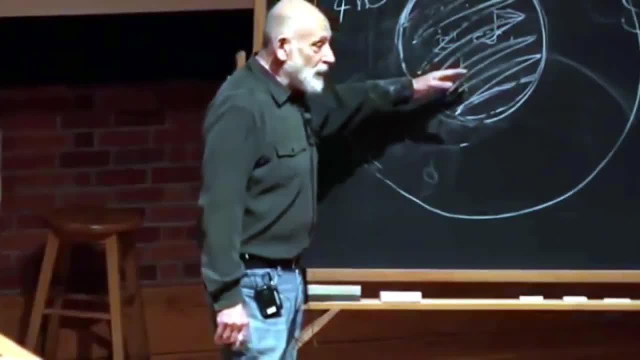 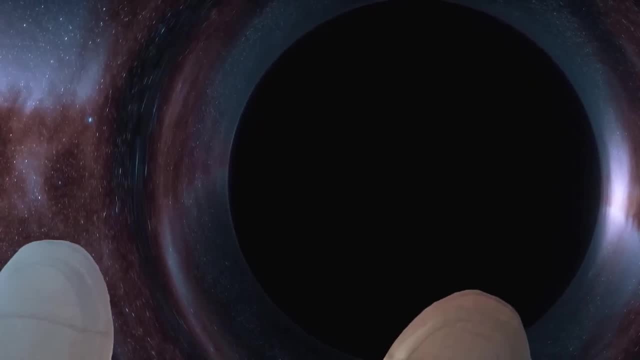 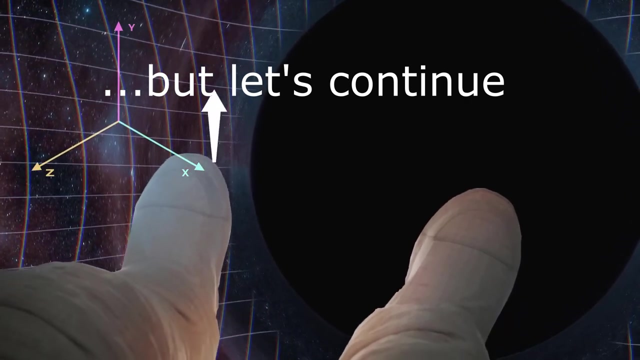 of jumping in the black hole. I think you would tell me: well, get me the black hole and you try it. But you know it's a problem. I don't know the answer In a non-expanding universe devoid of gravitational forces. 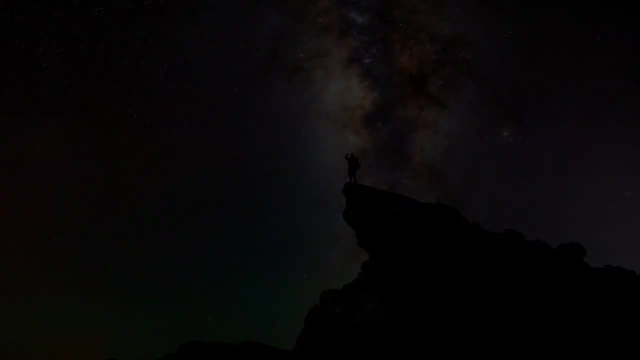 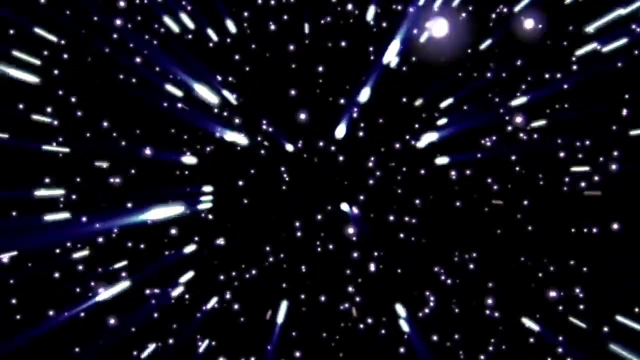 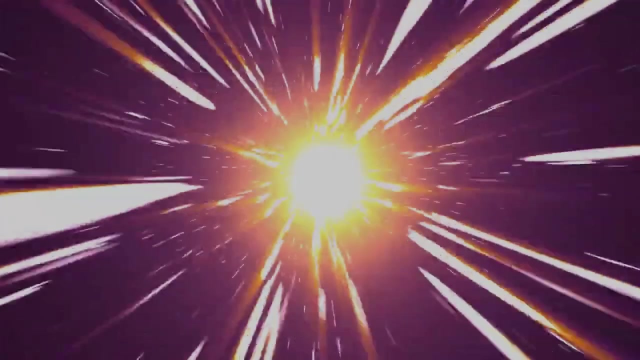 if a particle is moving at a constant speed, at a constant velocity, it will eventually be able to observe any event that takes place in that universe. This is because the forward light cones originating from these events cross with the particle's world line. Conversely, when the particle is undergoing acceleration, 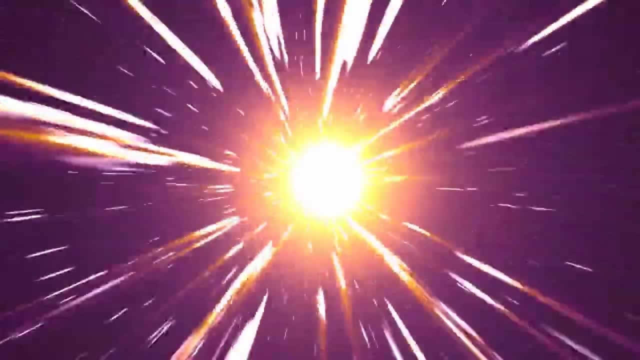 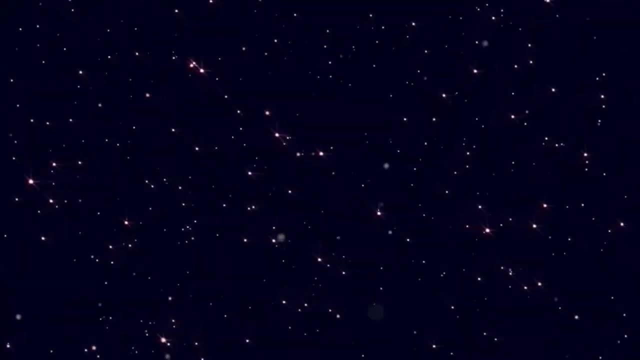 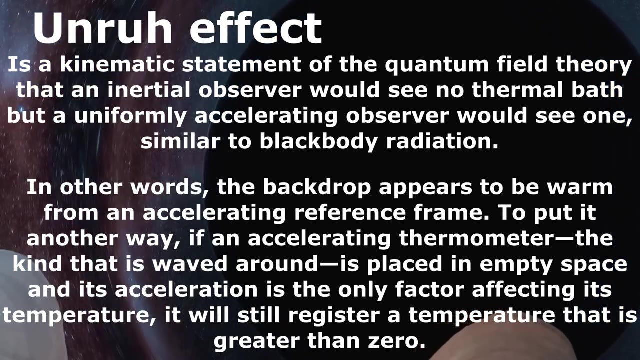 there are certain scenarios where the light cones of certain events do not cross with the particle's path through space-time. In these circumstances, a visible border, known as an apparent horizon, exists in the reference frame of the particle, indicating a limit beyond which events cannot be observed. 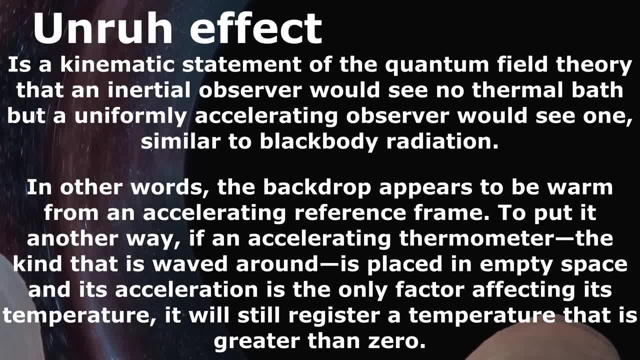 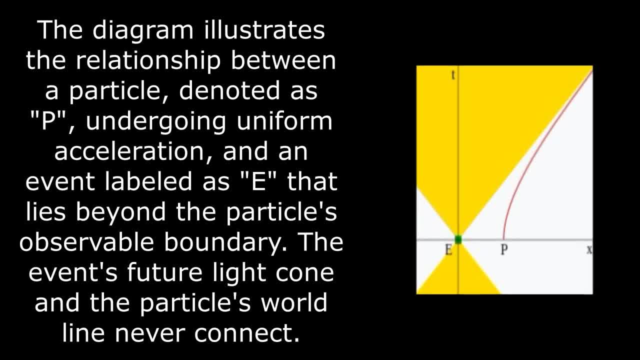 For instance, this phenomenon arises when dealing with a particle undergoing uniform acceleration. The picture to the right displays a space-time diagram of this situation. As the particle accelerates, it progressively gets closer to, but never attains the speed of light in relation to its initial frame of reference. 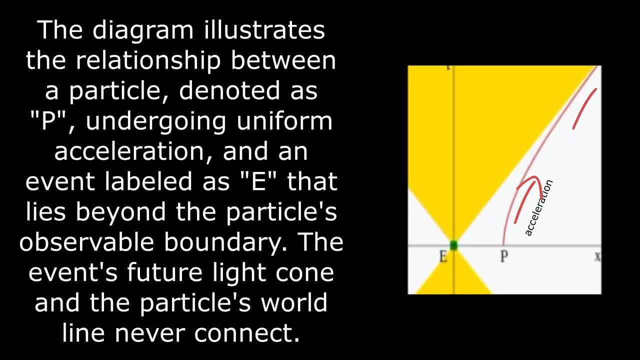 The root of the object on the space-time diagram is represented by a hyperbola that gradually approaches a 45-degree line, which corresponds to the path of a light beam, An event that lies beyond the asymptote or lies outside the light cone's border. 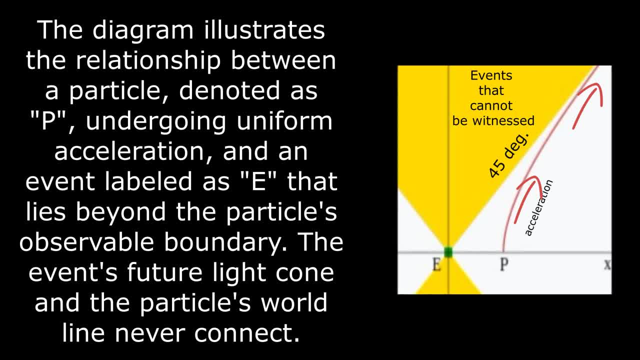 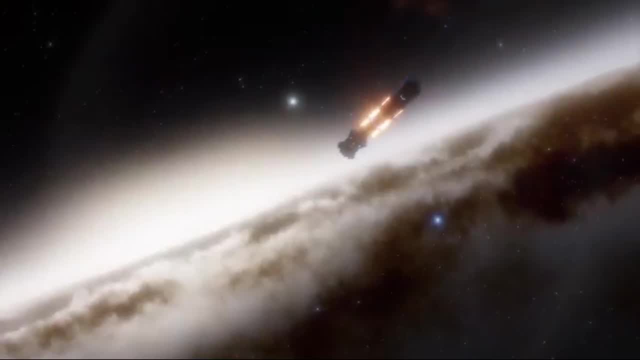 cannot be detected by the accelerating particle. Within the particle's frame of reference, there exists a limit located behind it, known as an apparent horizon, from which no signals are able to escape For an observer who is uniformly accelerating in empty space. 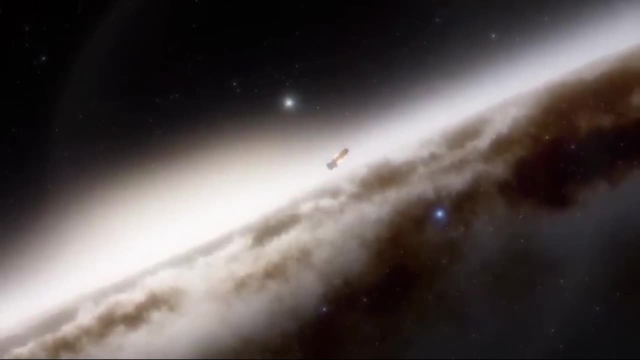 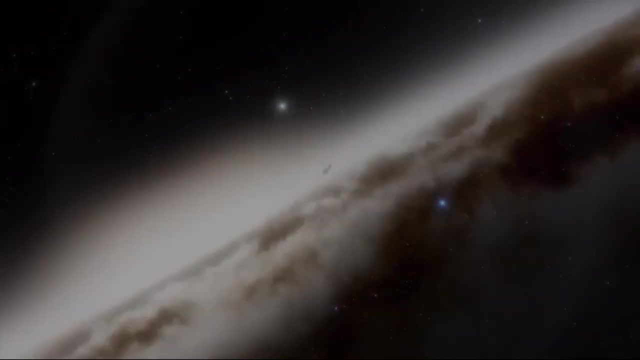 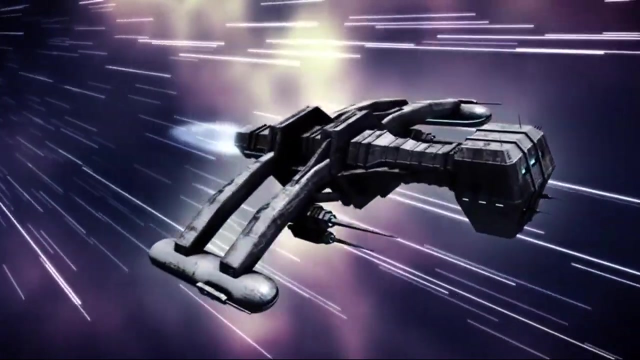 the horizon appears to maintain a constant distance from the observer, regardless of the movement of its surroundings. Modulating the observer's acceleration can result in the perception of the horizon undergoing motion over a period of time, or perhaps impede the existence of an event horizon. 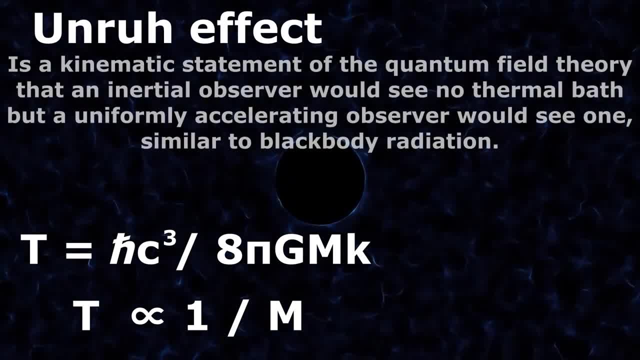 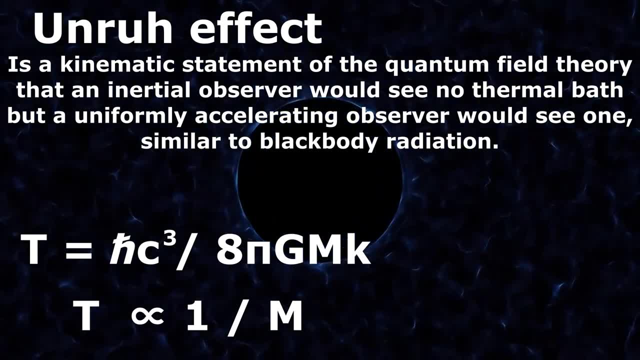 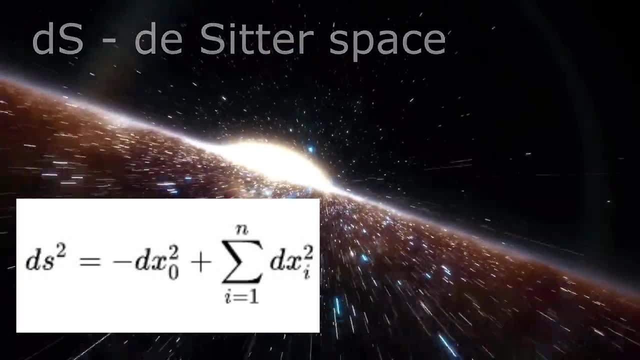 contingent upon the selected acceleration function, The observer remains continuously distant from the horizon and never traverses a point where it previously appeared. In the context of a de-sitter universe, the horizon is consistently viewed as being at a constant distance by an observer who is not undergoing any acceleration. 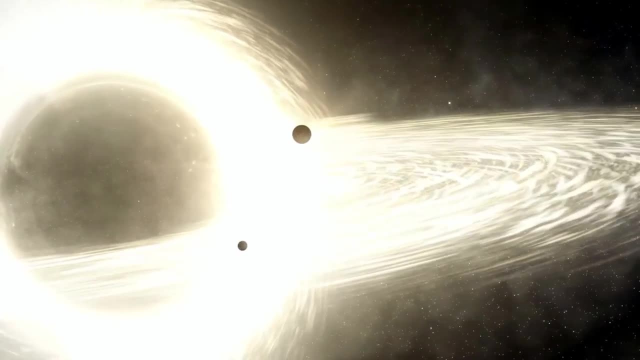 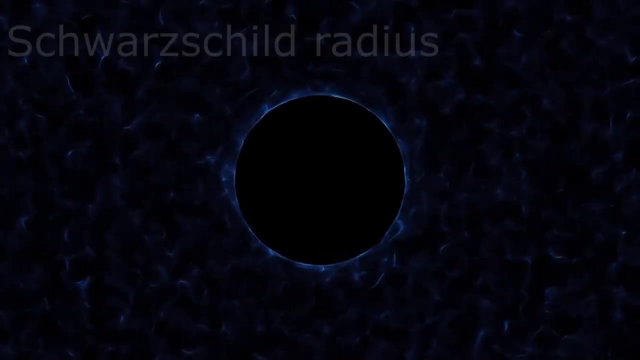 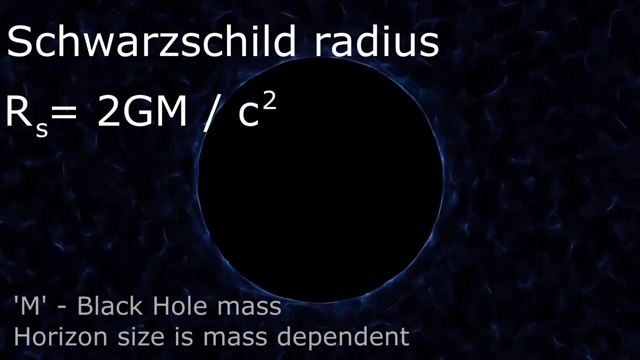 An accelerating observer never makes contact with it. An event horizon is a well-known concept in general relativity that arises from the description of a black hole. A black hole is an extremely massive astronomical object that exerts such a strong gravitational pull that no matter or radiation in its vicinity can escape. 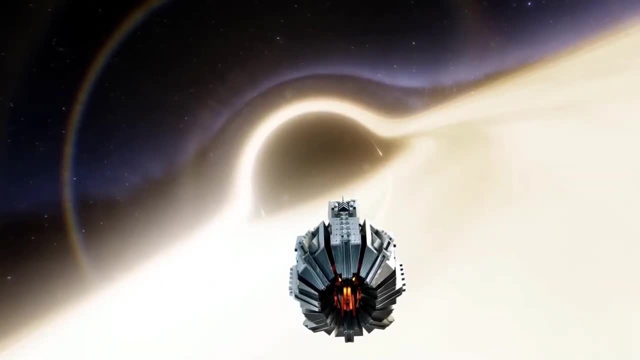 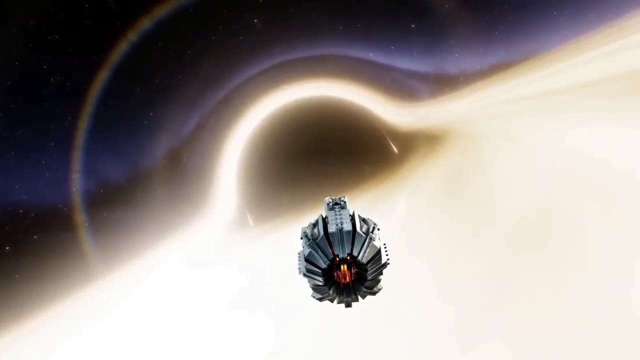 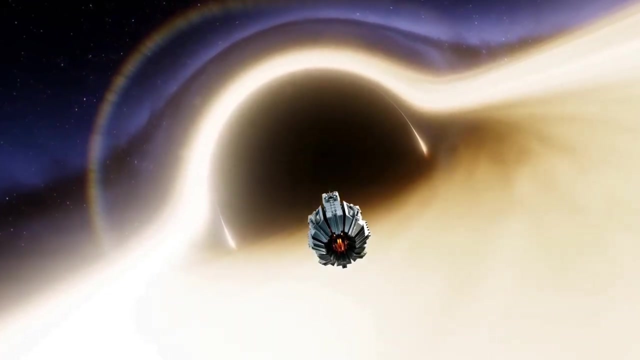 Commonly, this is referred to as the region where the escape velocity of a black hole exceeds the speed of light. However, to provide a more precise explanation, it may be stated that within this boundary, known as the horizon, all courses that light could potentially take. 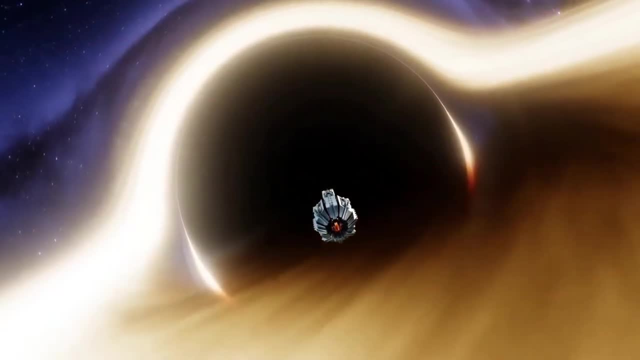 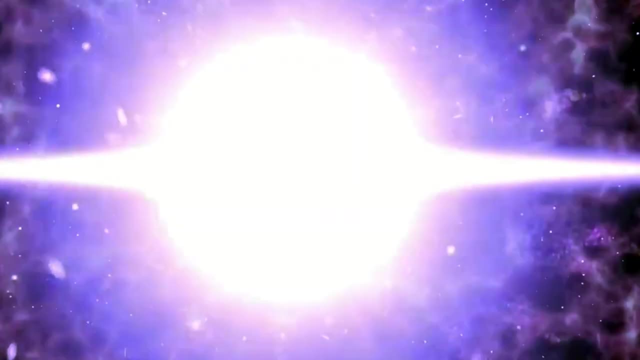 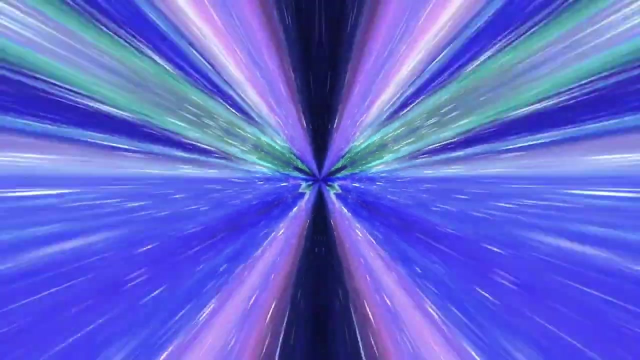 as well as all paths within the forward light. cones of particles located within the horizon are distorted in a manner that causes them to move farther towards the center of the black hole. Once a particle crosses the event horizon, its movement towards the black hole becomes unavoidable. 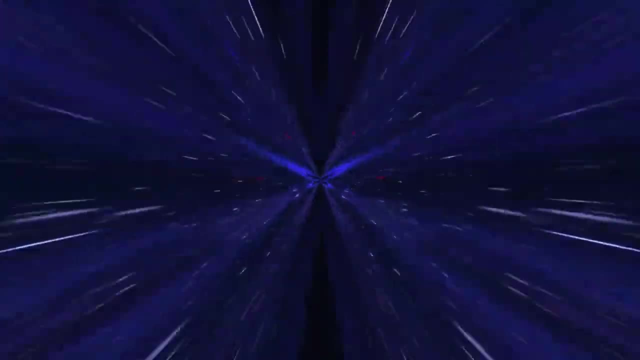 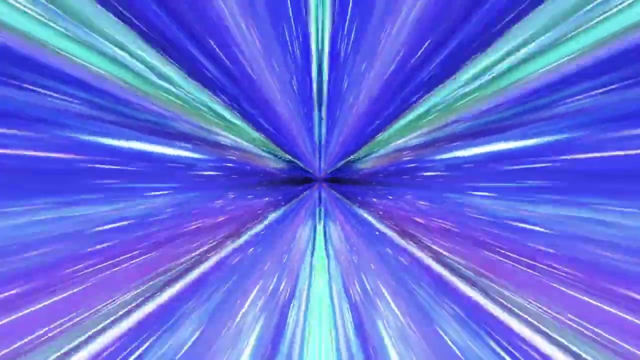 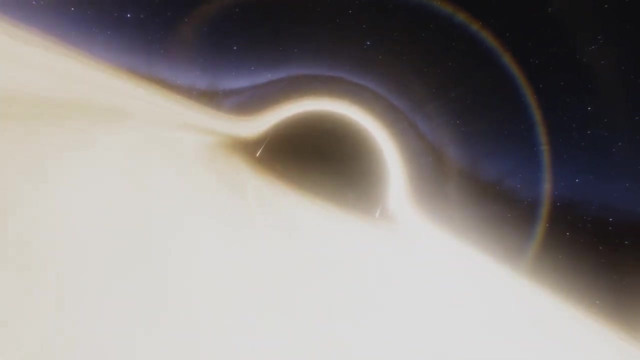 similar to the progression of time. This is true regardless of the particle's direction of travel and can be considered equivalent depending on the coordinate system used to describe space-time. An erroneous belief regarding event horizons, particularly those of black holes, is that they constitute an unchanging boundary. 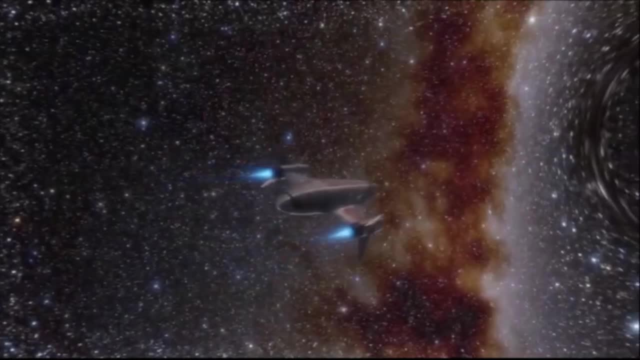 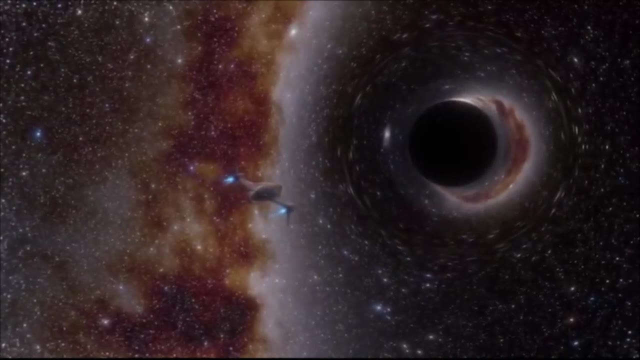 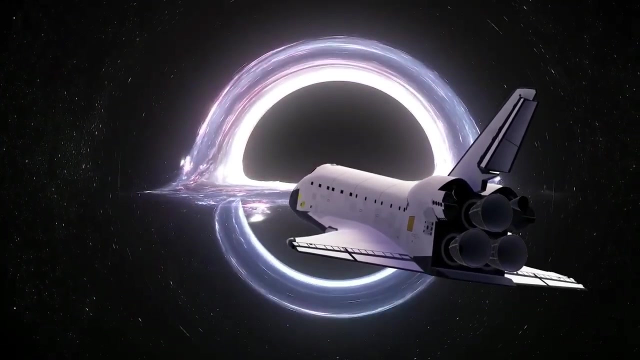 that annihilates things that come near them. In reality, event horizons always seem to be located at a certain distance from any observer. When objects are sent towards an event horizon, they never seem to actually cross it from the perspective of the observer who sent them. 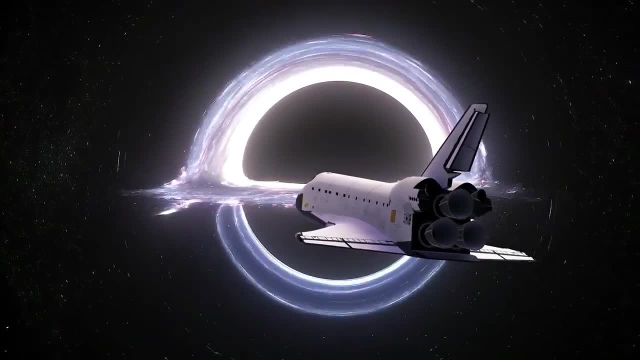 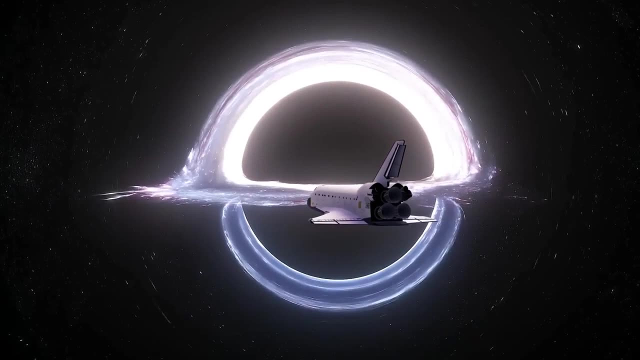 This is because the light cone of the event where the horizon is crossed never coincides with the observer's path through space-time. In order to keep an item located close to the horizon from moving in relation to an observer, an ever-increasing force must be applied. 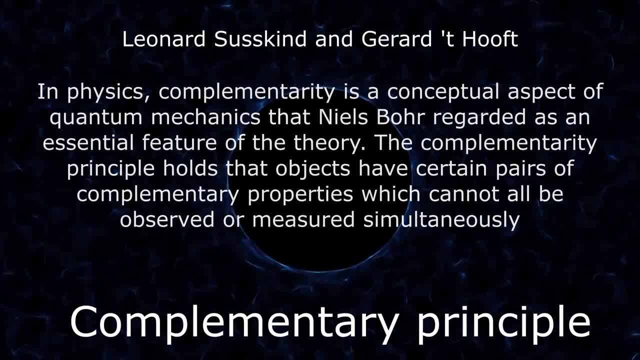 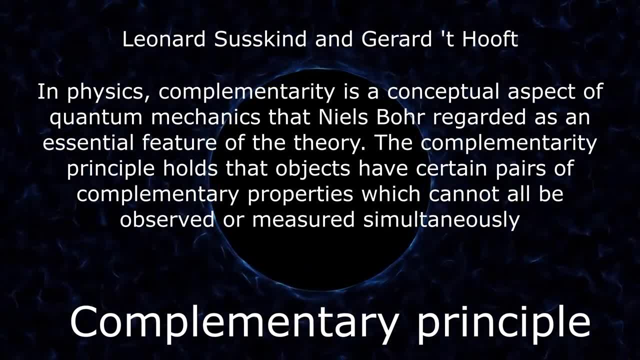 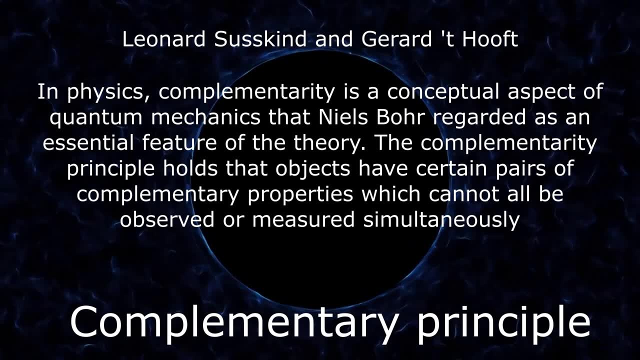 reaching an infinite magnitude as the object approaches. A cosmic event horizon is widely acknowledged as a genuine event horizon, Although the depiction of a local black hole or a small event horizon provided by general relativity is deemed incomplete and subject to debate When the circumstances in which local event horizons arise. 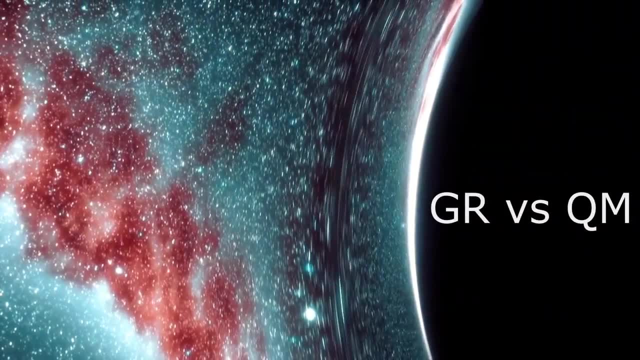 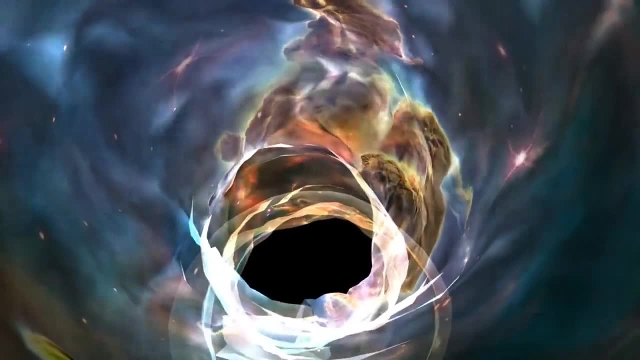 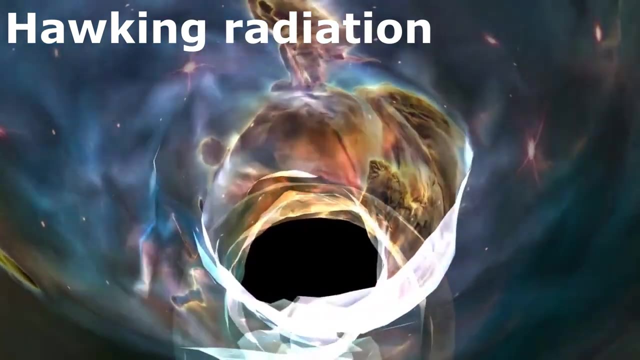 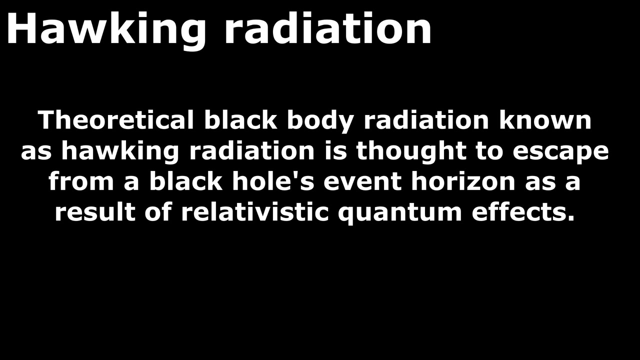 are simulated using a more inclusive framework of the universe's functioning, which incorporates both relativity and quantum mechanics. Currently, according to the Hawking radiation theory, quantum phenomena are anticipated to cause event horizons to have a temperature and also release radiation. Hawking radiation is a manifestation of black holes. 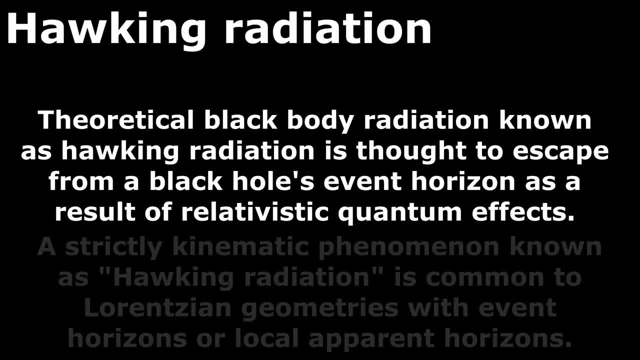 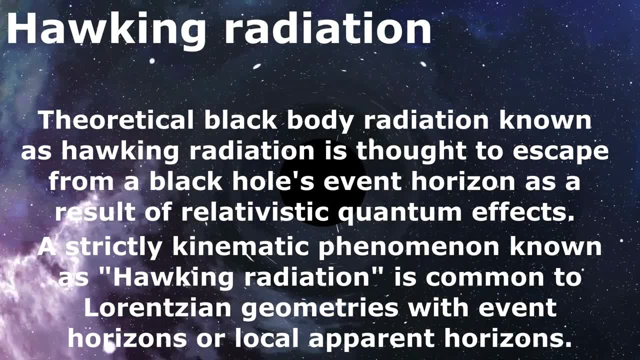 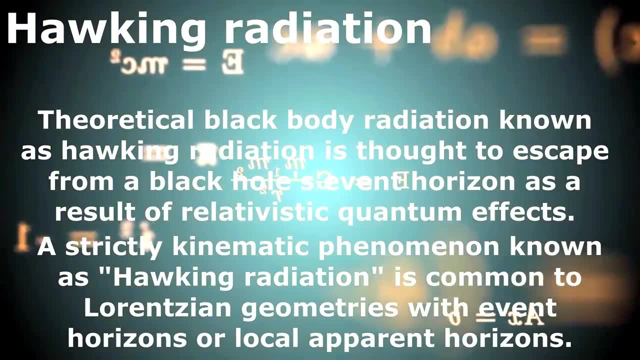 and the question of how black holes have a temperature is a key aspect of black hole thermodynamics. The acceleration of particles gives rise to the Unruh effect when the surrounding space seems to be filled with matter and radiation, As per the contentious black hole firewall idea. 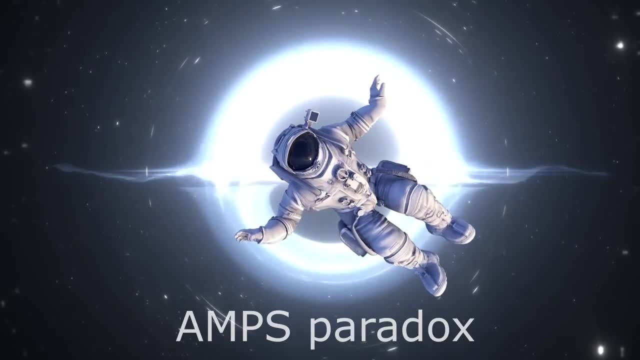 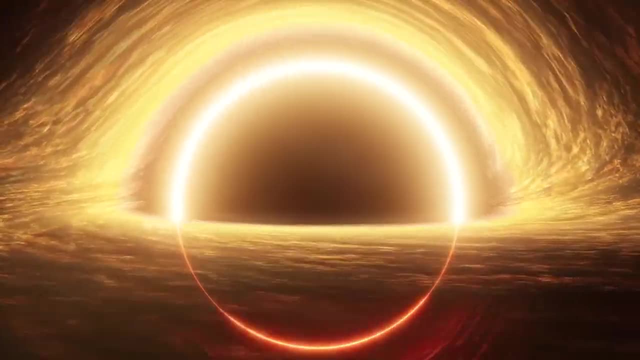 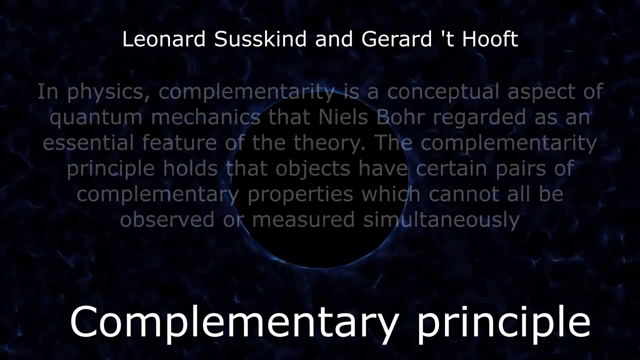 any matter that enters a black hole would be incinerated by an intense and energetic firewall located near the event horizon. The complementarity principle offers an alternative explanation. According to this principle, when observed from a distant point, matter falling into a black hole is heated up at the event horizon. 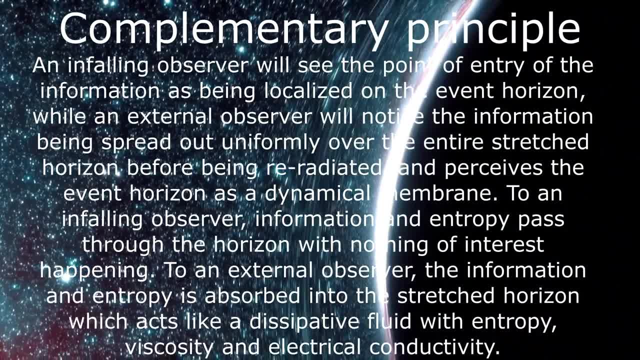 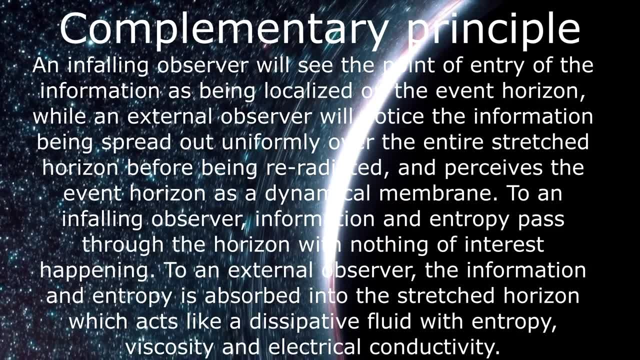 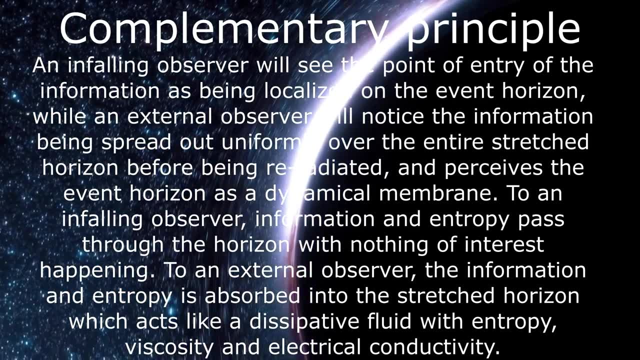 and then emitted as Hawking radiation. However, when observed from the perspective of an object falling into the black hole, the matter passes through the inner region without any disruption and eventually gets destroyed at the singularity. This hypothesis does not contravene the no-cloning theorem. 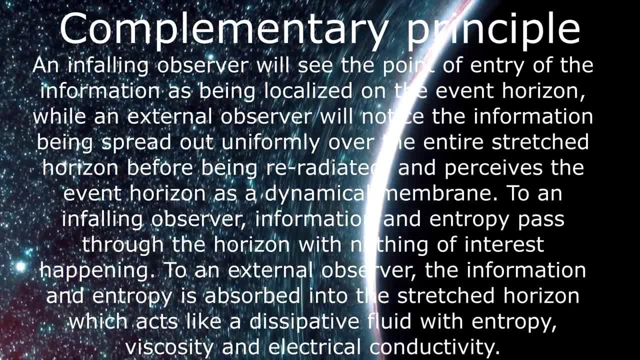 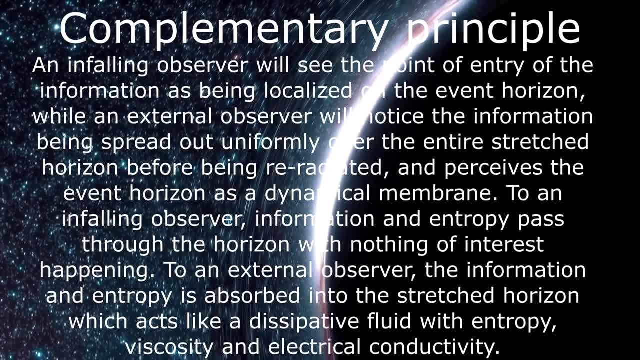 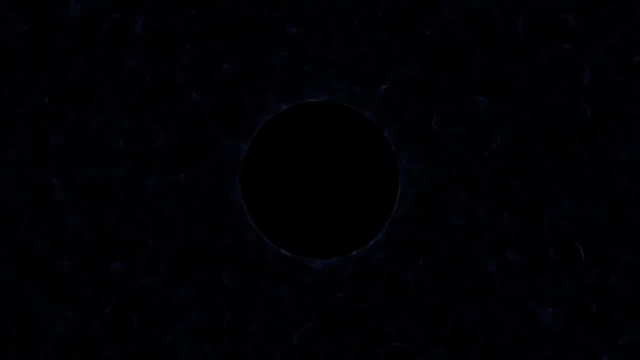 since there exists only one instance of the information as perceived by each particular observer, The concept of black hole. complementarity is proposed, based on the scaling laws of strings as they approach the event horizon. These laws indicate that in the Schwarzschild chart, the strings extend to encompass the horizon. 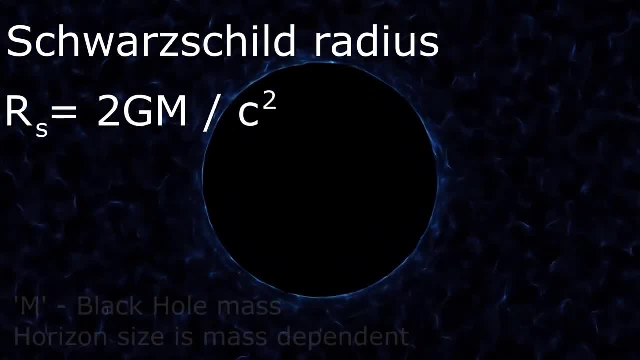 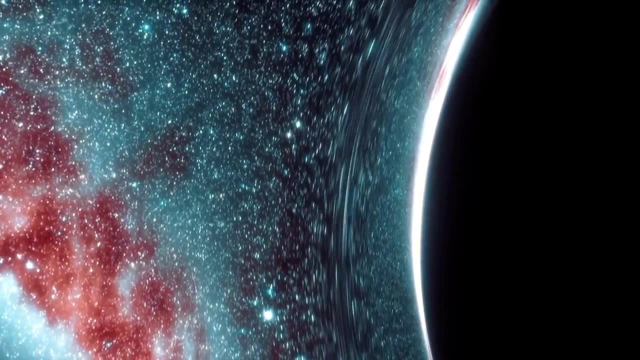 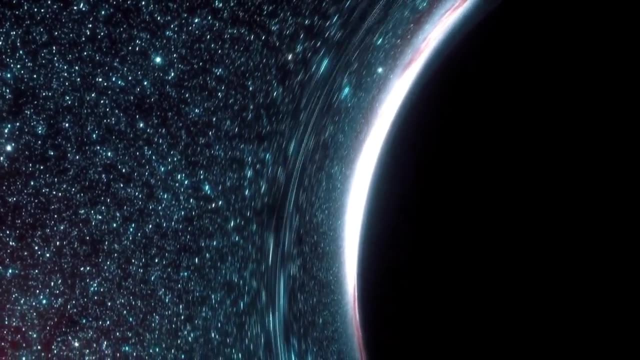 and transform into a membrane with a thickness equivalent to the Planck length. A comprehensive explanation of local event horizons produced by gravity necessitates, at the very least, a theory of quantum gravity. Currently, a quantum theory of gravity is not on the table. 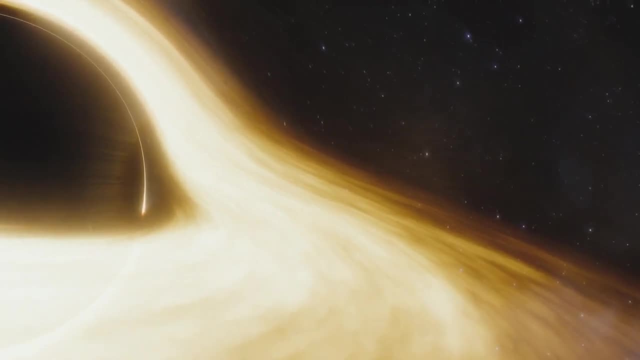 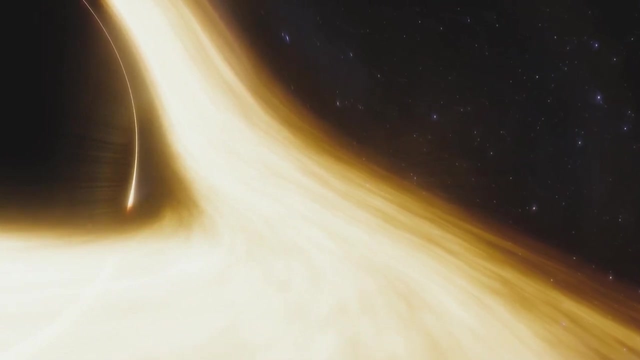 although promising steps towards it have been made within the context of entanglement and wormholes, the two sides of the same phenomenon, Advances in quantum computing is expected to shed light on nature of gravity itself, because a quantum computer is one for which the particular effects of quantum gravity are relevant. 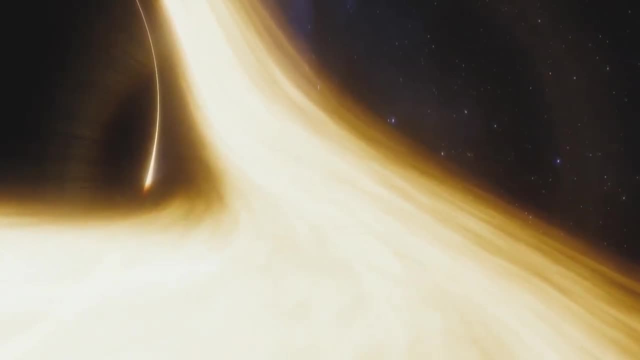 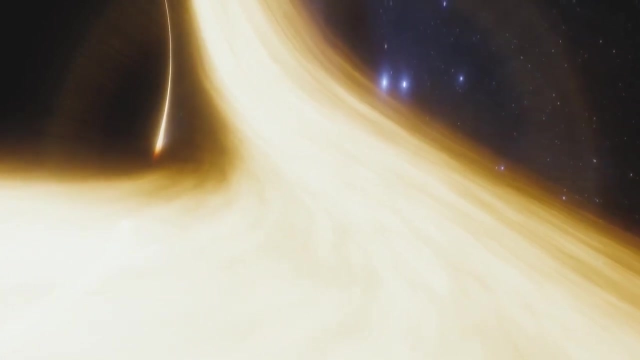 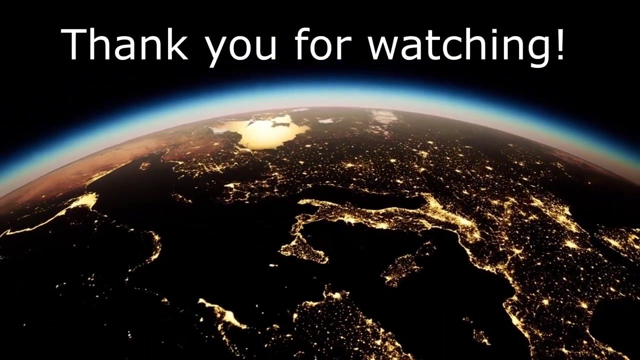 I will stop here for the moment. We will continue this discussion in another video. For now, I believe the event horizon presentation was comprehensive enough for everybody to understand. Thank you for your attention. If you have any questions or comments, please post them in the comments below. 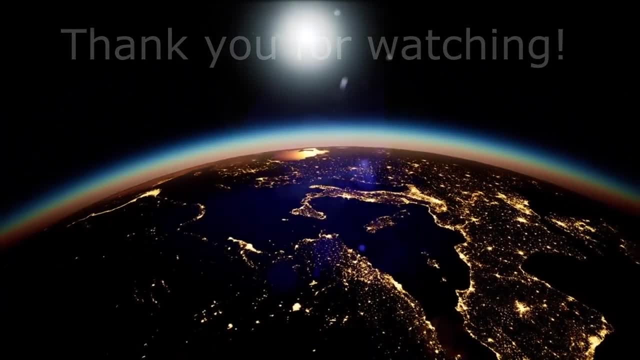 Thank you for your attention. Thank you for your attention.